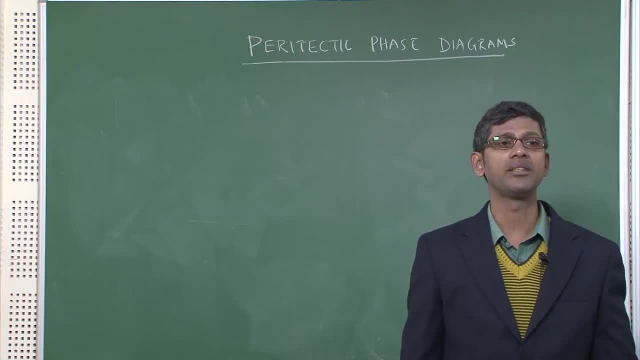 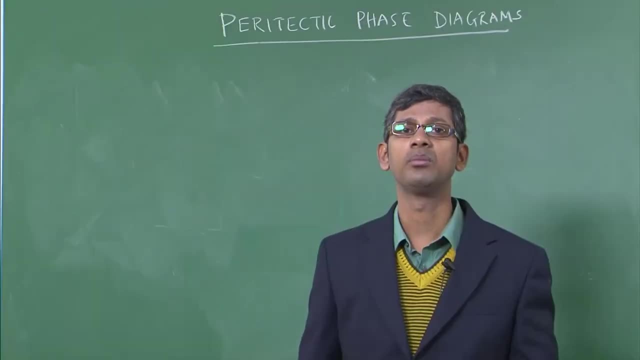 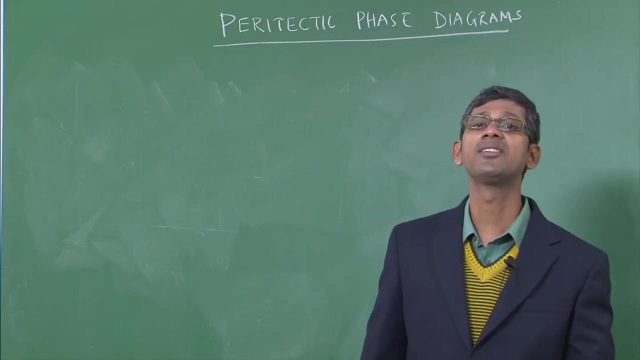 system. There are about more than 5 peritectic reactions present in the copper and zinc system. Similarly, bronze, copper and tin- an alloy- has peritectic reactions. Similarly, many, many industrial important alloy- let us think of iron and carbon. classical steel has peritectic 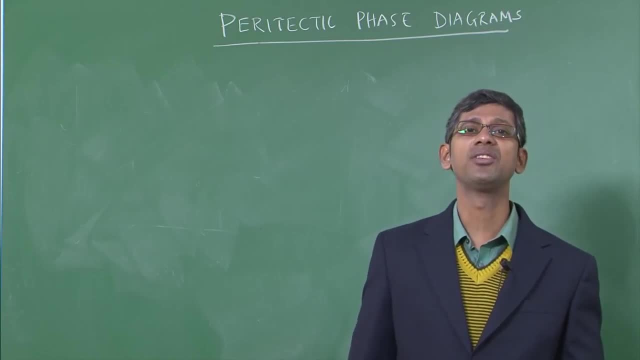 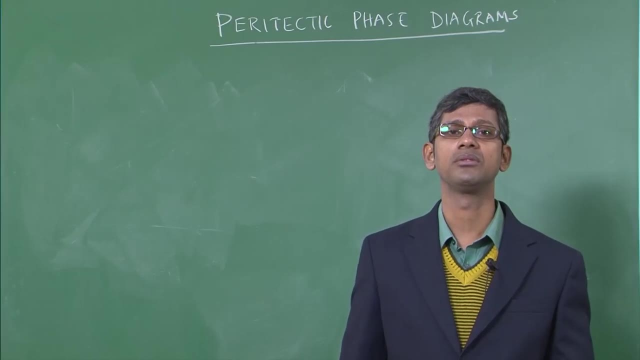 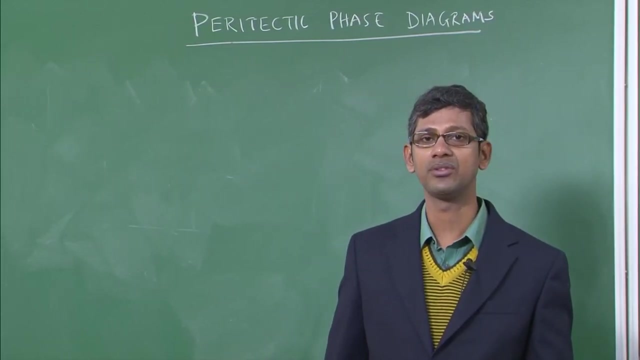 reactions And peritectic reactions. for the steel lies very low carbon concentrations, as about 0.13 percentage of carbon, So that means that peritectic reaction is very general in the phase diagrams And many ceramic system also has peritectic reactions, like all the superconducting material. 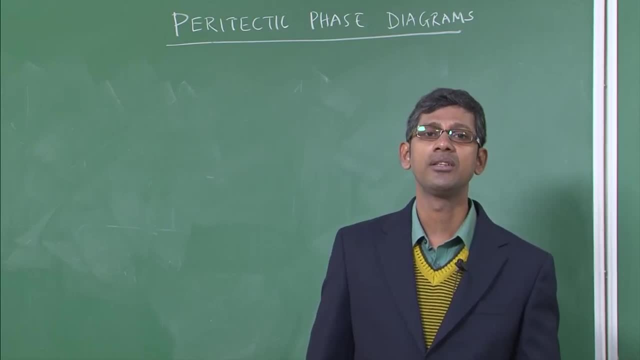 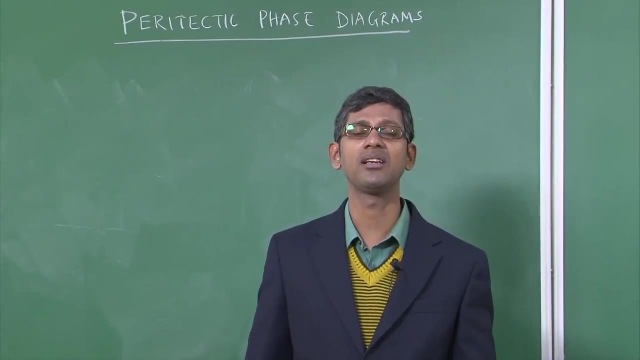 many of these has a peritectic reaction present. That's why it is very important so that we understand the peritectic phase diagram and the solidification. In the first lecture I will just try to explain the phase diagram and show you how the things 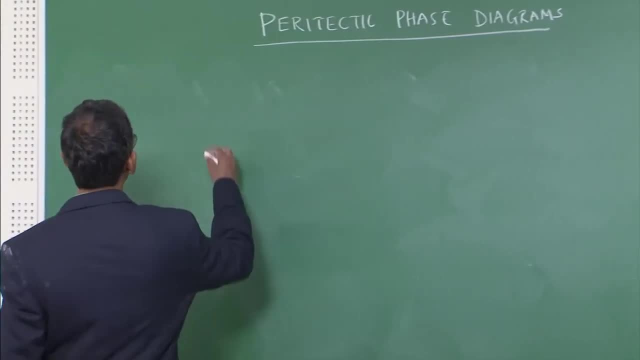 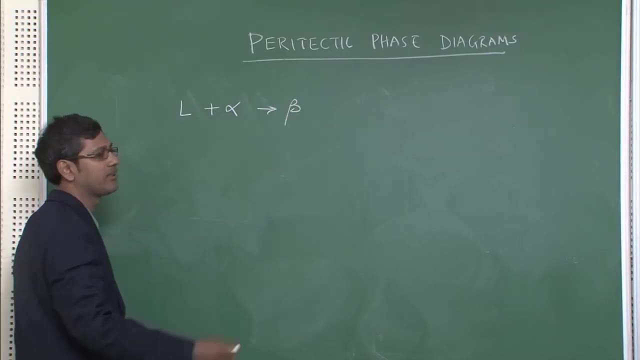 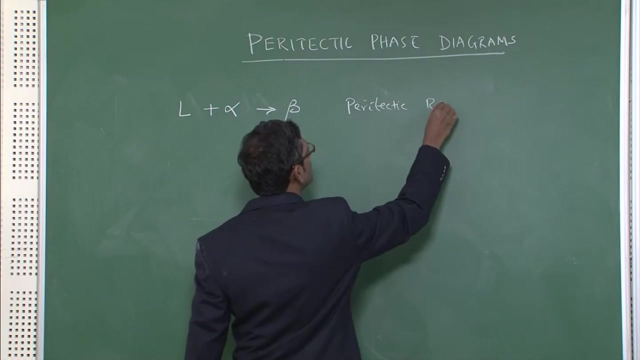 occur. So classical peritectic reaction is given by liquid reacting with a solid phase giving rise to another solid phase. This is a peritectic reaction. This is a very important reaction, allocating log of both the phase components. smartest in ocean being found, ones must strong. 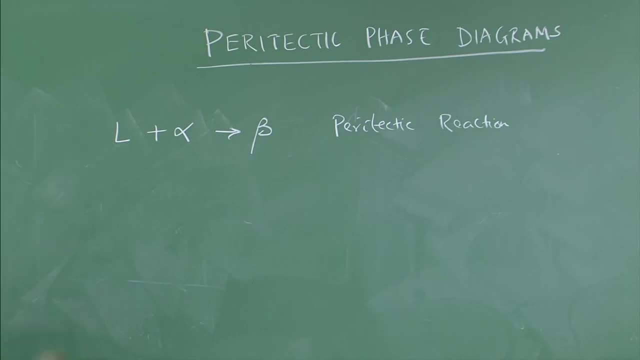 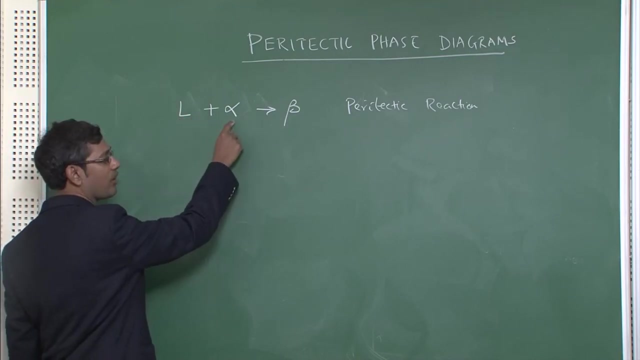 YinLook. so basically otherates Basket, a possible number of alloys. 그런데 this Gum, these are alloy development depends on this reaction. So please try to understand that here. one liquid phase reacts with another solid phase. one solid phase leads to formation of another solid phase. 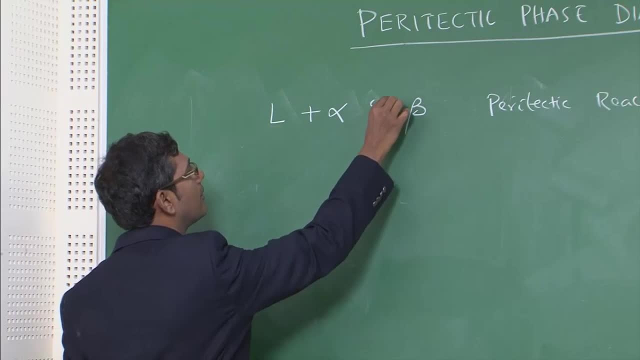 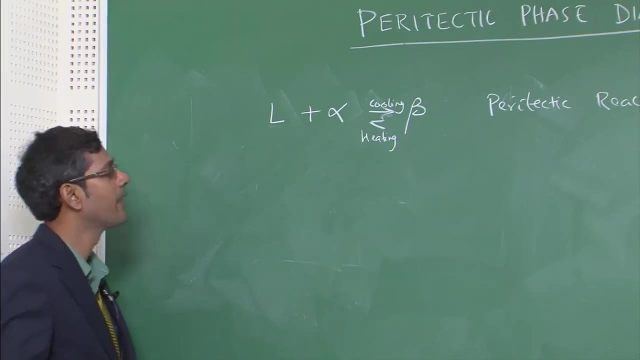 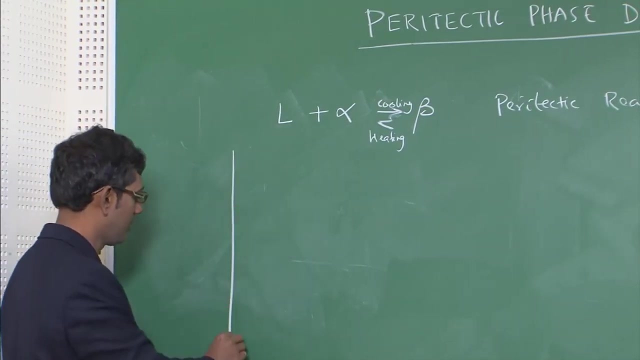 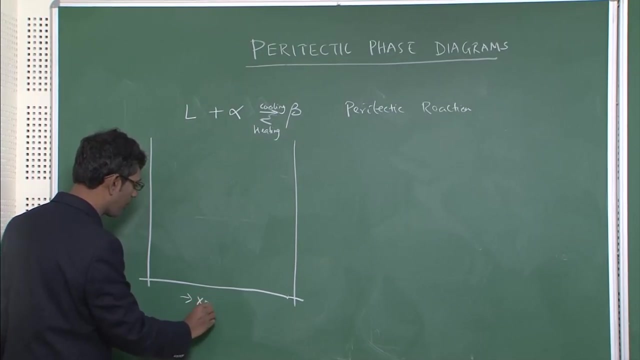 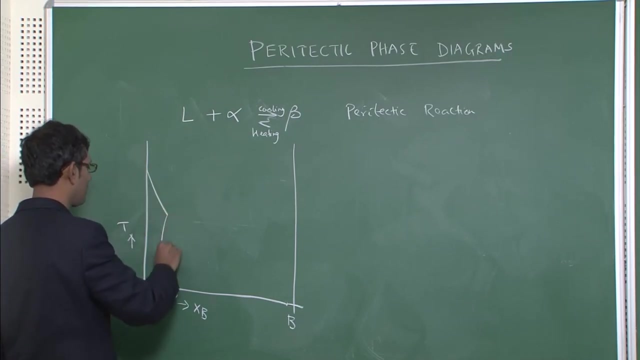 Sometimes it is written like this: during cooling it will form beta. during heating beta will dissociate into solid and liquid. So this kind of reaction can be represented in a phase diagram in this way. Again, I draw: the composition exists first, pure A, pure B. ends temperature: 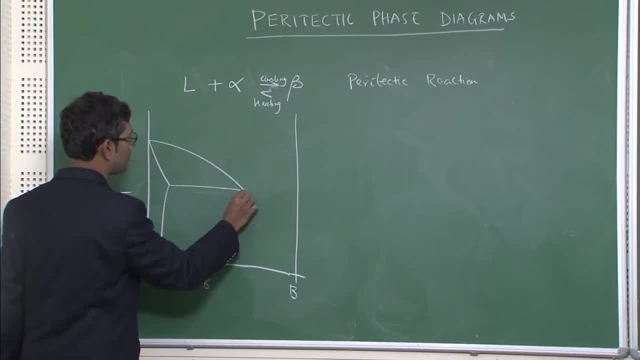 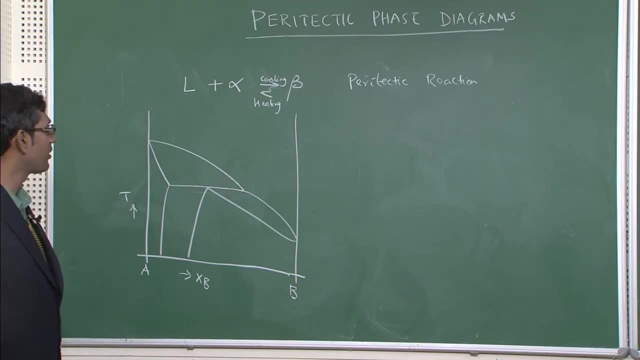 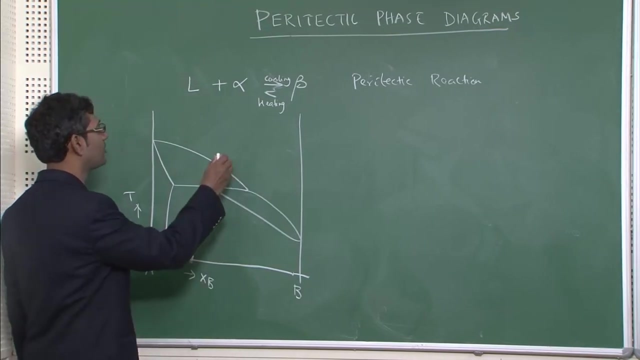 Okay. Okay, So this diagram is completely different from eutectic. In eutectic phase diagram I have seen there is a dip at the center. here it is not present. So this is pure liquid. this is the melting temperature pure. A melting temperature- pure. 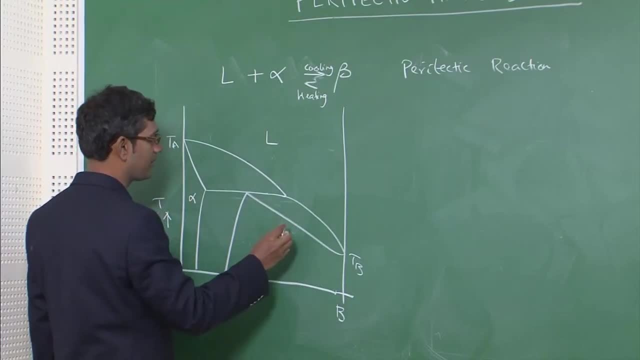 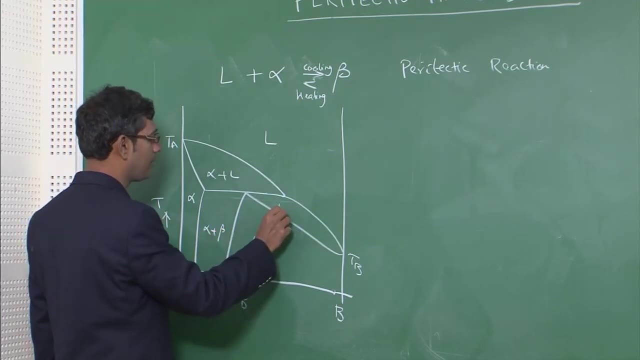 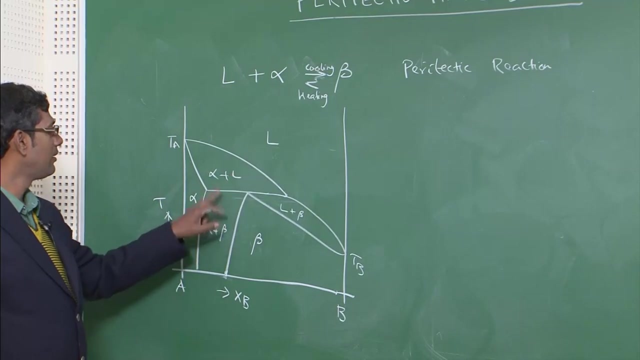 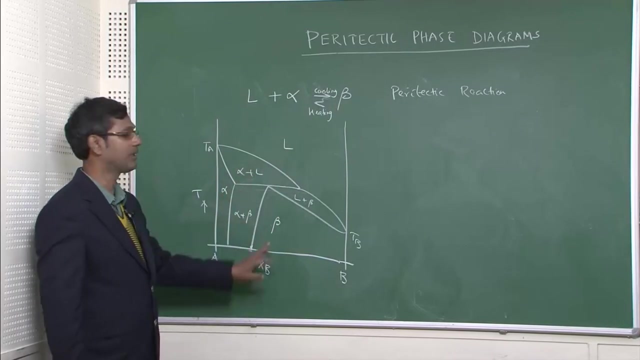 B, alpha. This is alpha plus liquid, this is beta, alpha plus beta. So you can clearly see again. there are three two phase field liquid plus alpha, liquid plus beta, alpha plus beta and three solid phase field liquid- alpha, beta. 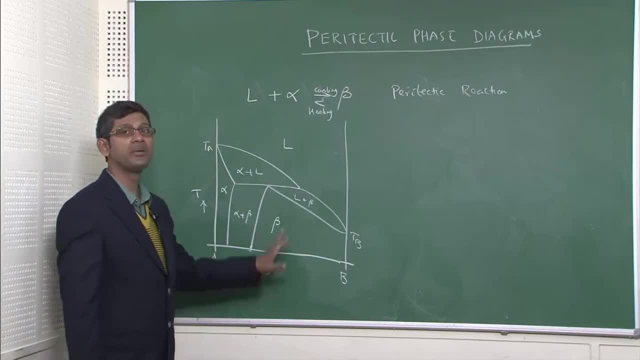 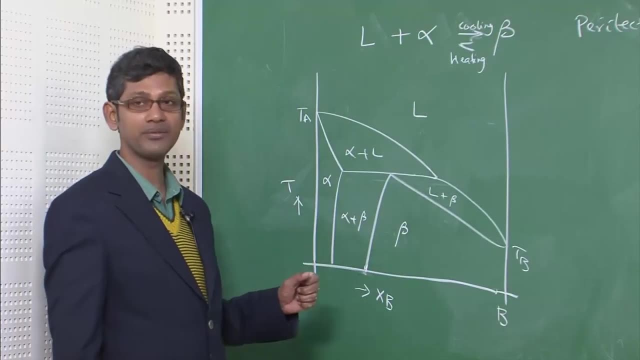 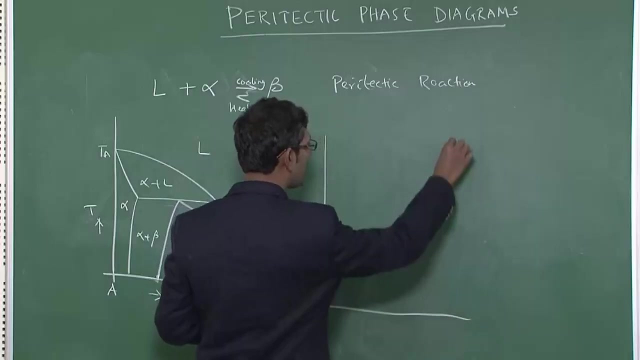 Same like eutectic systems, but the diagram is completely different. In fact this is not easy to draw. Sometimes students face difficulty in drawing the phase diagram. So I, for generalization, I am just drawing the phase diagram of eutectic here so that you can keep it in. you can keep. 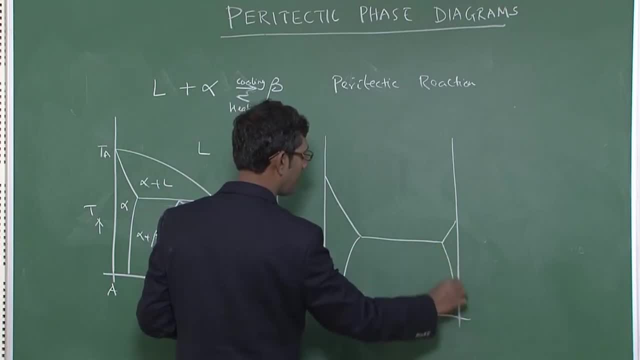 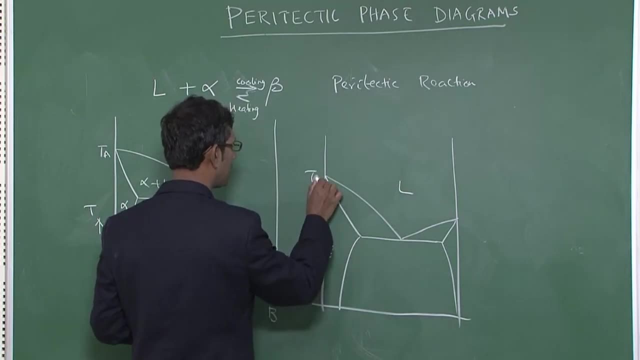 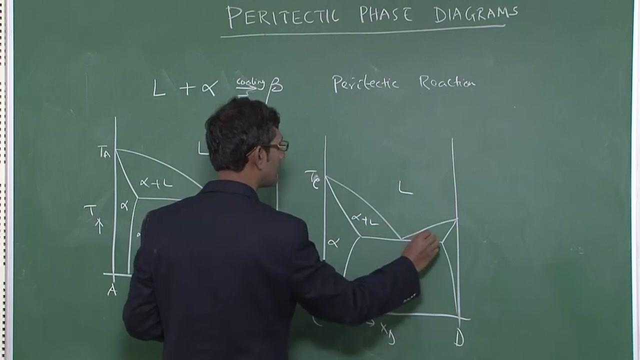 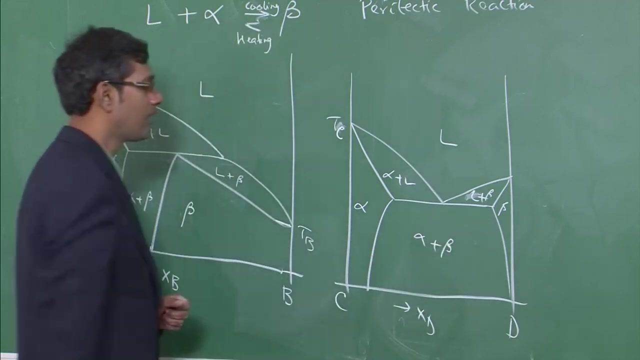 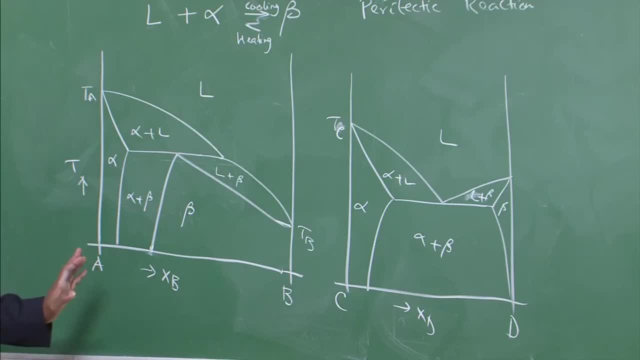 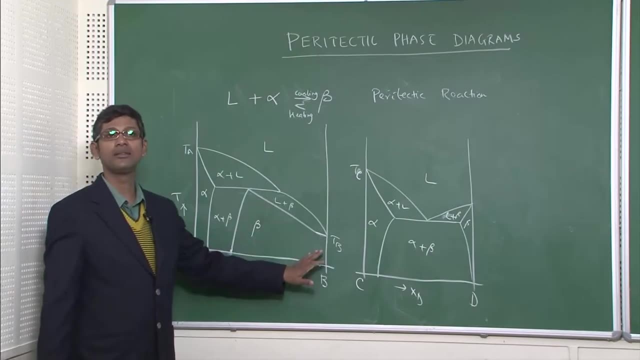 Okay, Very good. So this difference, So this difference is very clear, Very clear. So you can clearly see the difference. It is not at all looking very similar, Rather it is different, Distinctively, it is different. So these kinds of phase diagrams actually observed for systems when you have a large 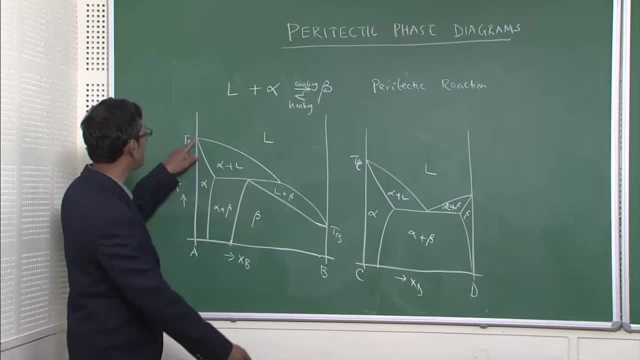 difference in melting temperatures between A and B. as you can see, as TA is here, TB is there, Melting temperatures of A and B are large difference. So whenever you have such a kind of large difference of melting temperatures and we 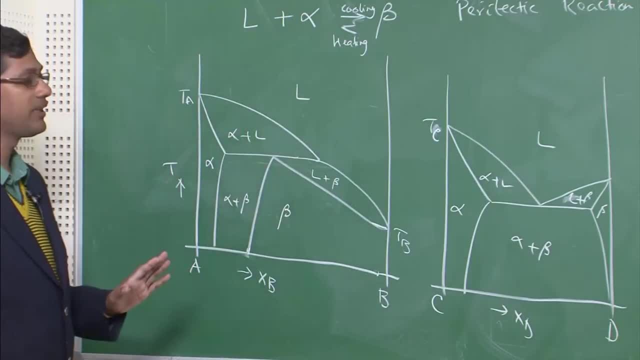 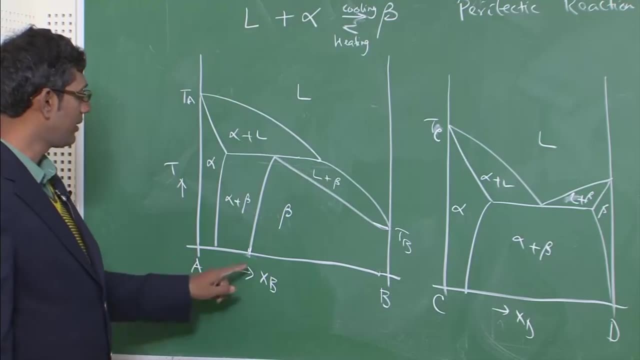 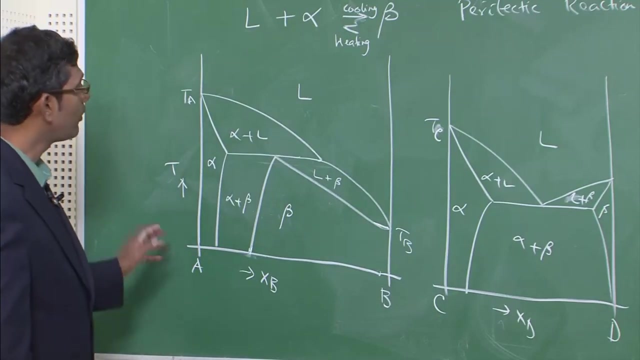 can call that inzinhof. That is the difference between the different surrounding states, Anon, Sure, and interaction between A and B, which we will discuss later, is strongly negative. then you have this kind of phase diagram formations. So let me just discuss about this phase diagrams in little detail manner. 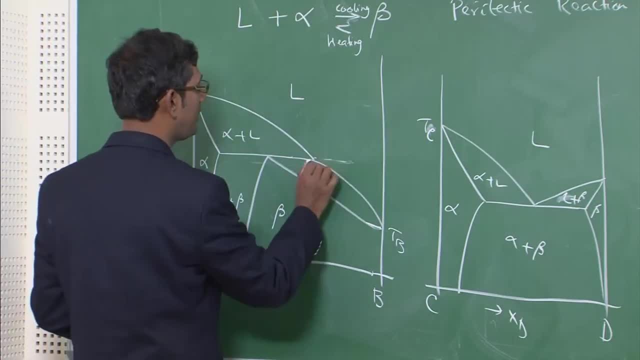 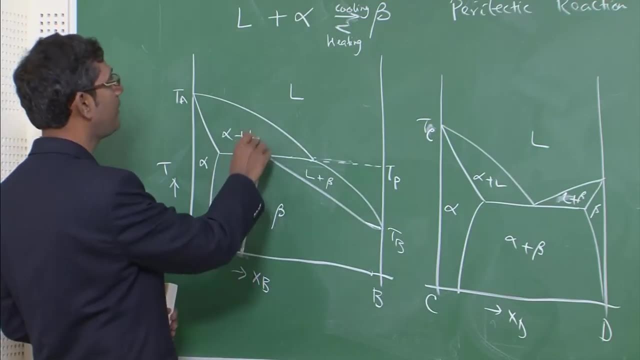 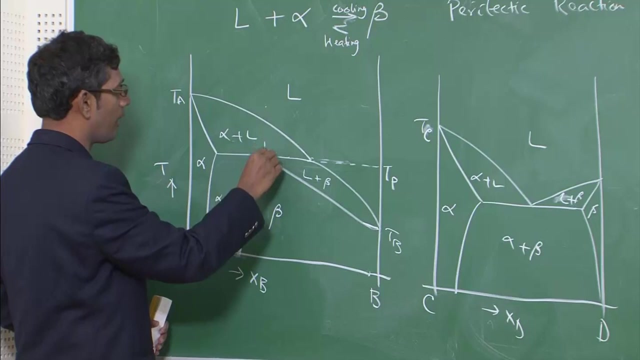 Here the p-tree reaction happens at a temperature known as Tp. this temperature and reaction is taking place here, in which alpha plus liquid reacting with each other and forming beta. this is where- So if you cool down this one the way I have drawn the arrow, alpha plus liquid or liquid. 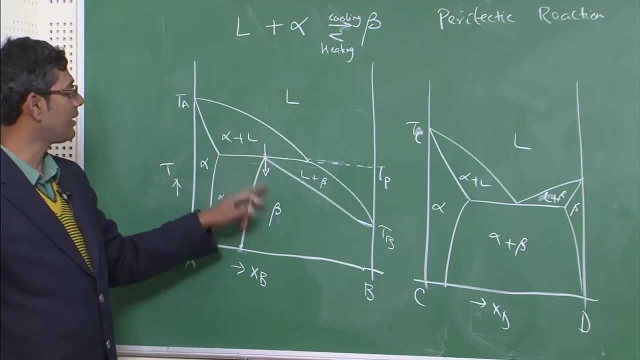 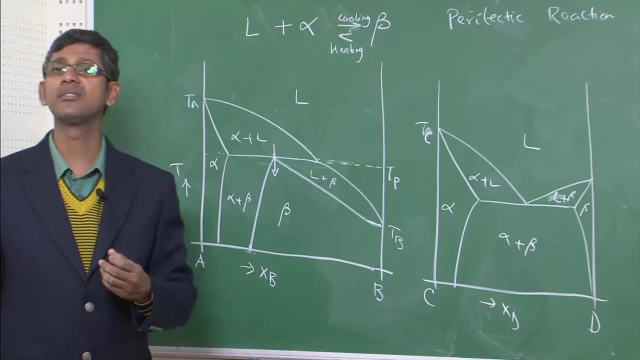 plus alpha- whichever way you say- reacts with each other and forms beta. this is where the reaction takes place. So this is a horizontal line. I told you as a thought that any horizontal line in a phase diagram will give you the reaction. 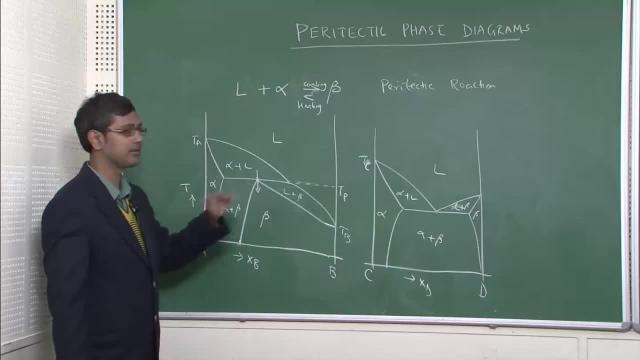 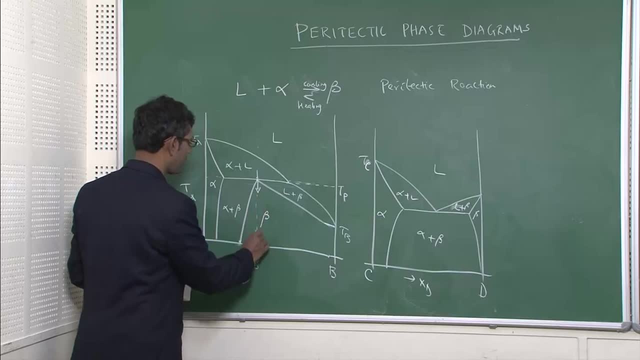 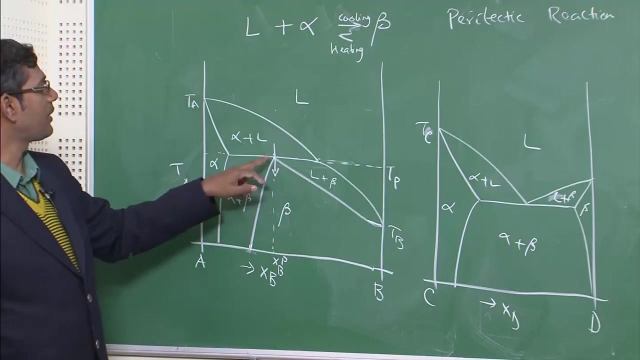 The idea of the reaction or some kind of reaction. So at this temperature, Tp, at the composition given by this which I can draw- this is Xp, Xbp- the reaction happens. So that means at this temperature, Tp and composition, Xp, alpha liquid and beta, three phases are. 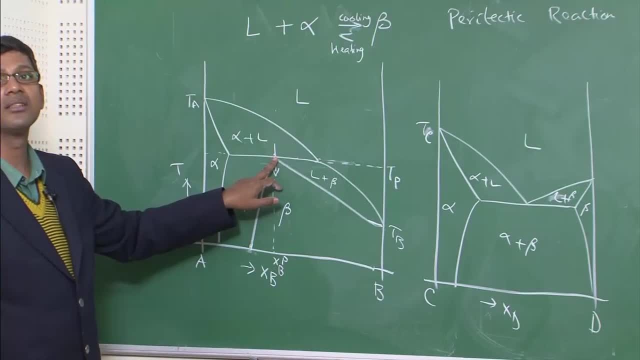 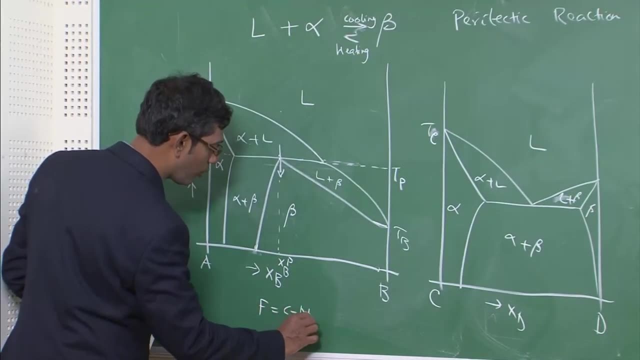 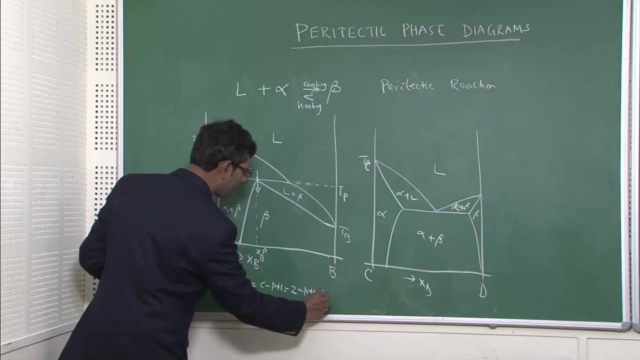 at equilibrium. so therefore degrees of freedom here is zero. Why degrees of freedom? Because we know degrees of freedom is given by C minus P plus 1, and here there are two components. so 2, C is 2, P plus 1, so 3 minus P. 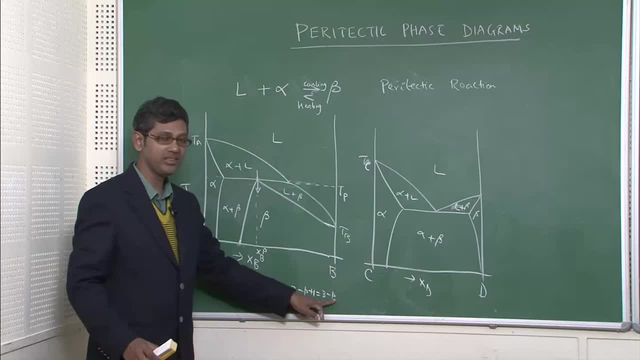 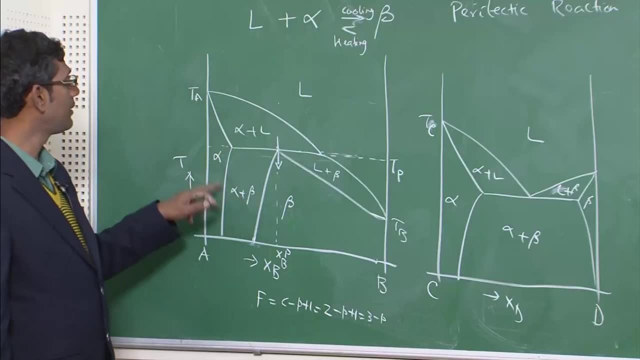 So if there are three phases present here, so 3 minus 3, P is 3, F becomes 0, so degrees of freedom is 0 at this point Now. similarly, in the two-phase field regions, where you have two phases, alpha plus beta. 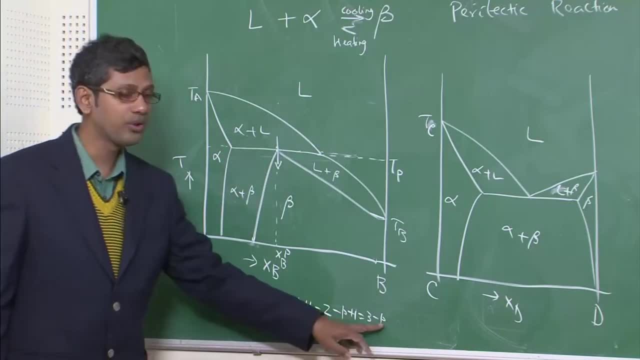 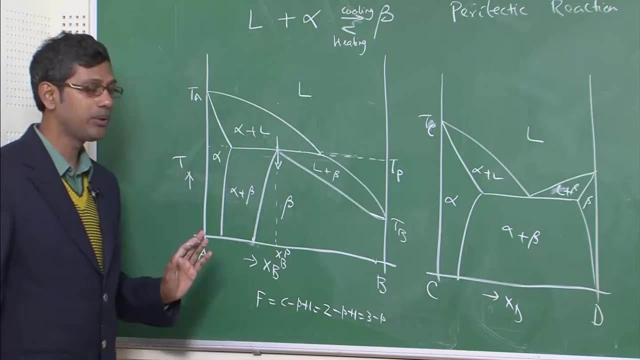 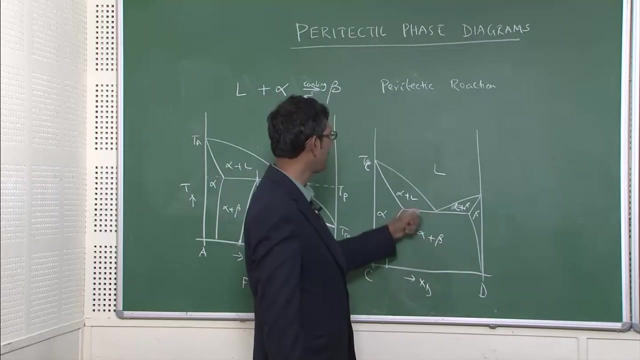 alpha plus liquid, beta plus liquid Degrees of freedom is equal to 1, and in the single-phase field, like beta, liquid or alpha degrees of freedom is equal to 2, okay, you remember. you should remember that Same thing here also: degrees of freedom at this point is 0 and here, there, there, degrees. 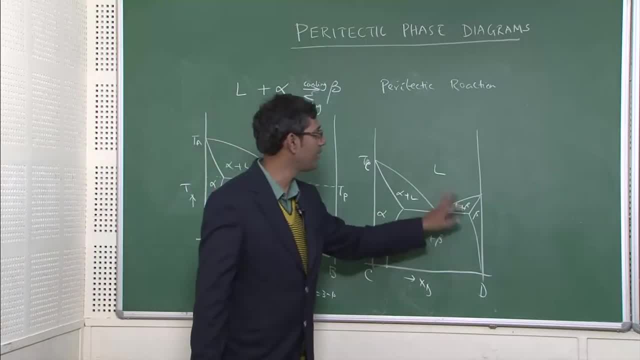 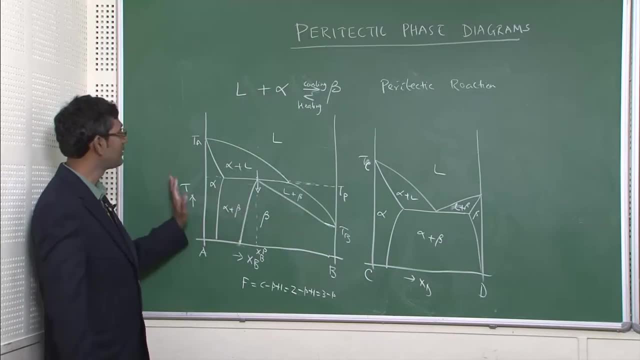 of freedom is equal to 1, other hand, in the alpha and beta and liquid regions, degrees of freedom is equal to 2.. So there is some similarity between these and these, but the inside diagram is completely different. This is the eutectic one. 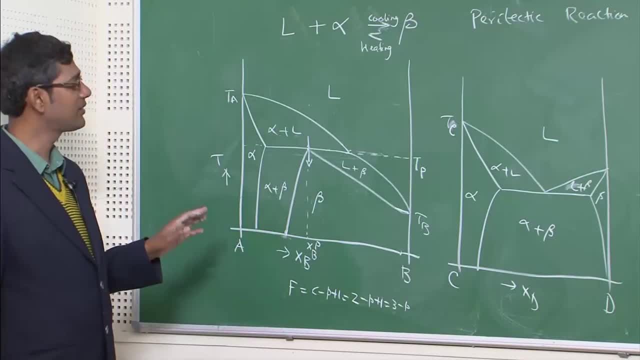 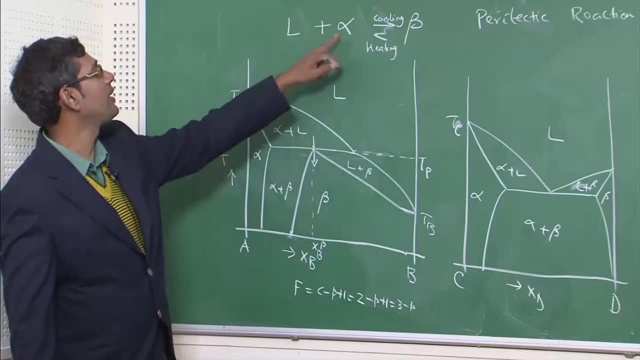 So now, upon knowing this, pectin reaction is distinctly different from eutectic. In eutectic reaction, two solid phases comes out from the liquid. Here, one solid reacts with the liquid, forms another solid. So therefore, this reaction is completely different. 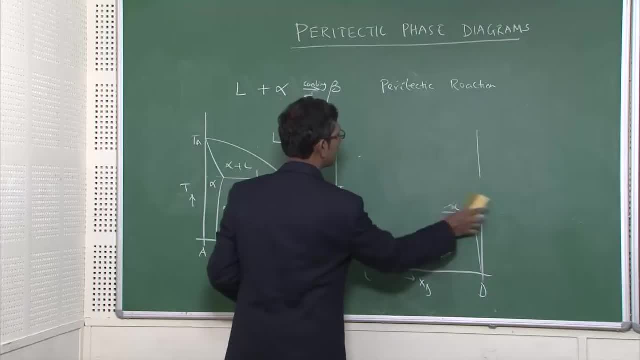 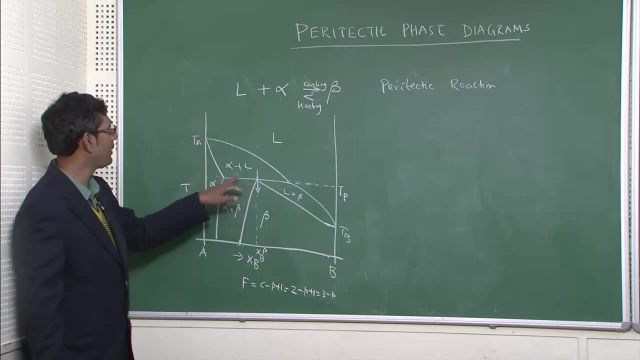 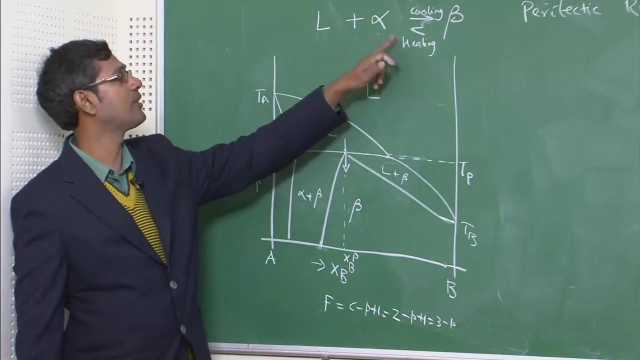 Now I will tell you why this reaction is completely different. okay, So let me just reiterate again. You have a pectin reaction, Pregnancy reaction, isotherm at temperature, Tp composition, Xpv enriched liquid reacts with alpha giving twice the beta. 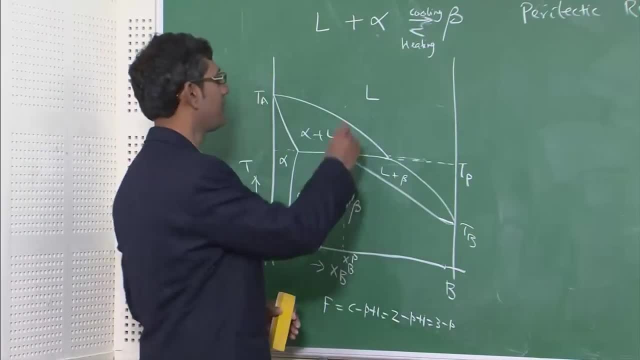 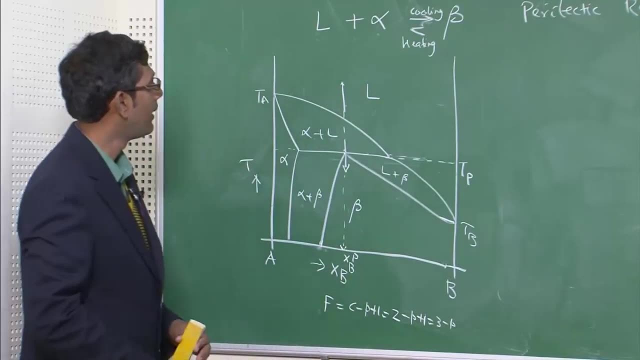 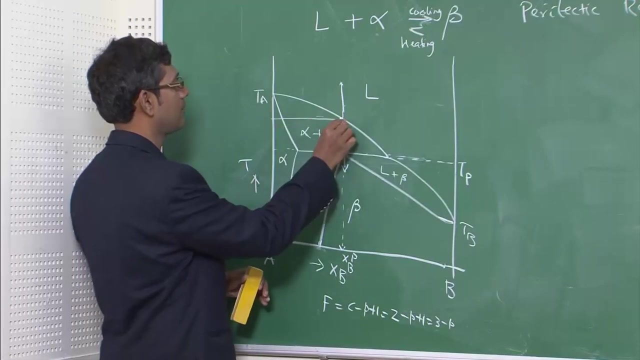 Now how does the reaction happens? Suppose I have an alloy which is certifying this composition Xpv from liquid state. So I am drawing this vertical line and I am following it up. So obviously, if I cool it down from liquid, this is my liquidus Tl, above liquidus everything. 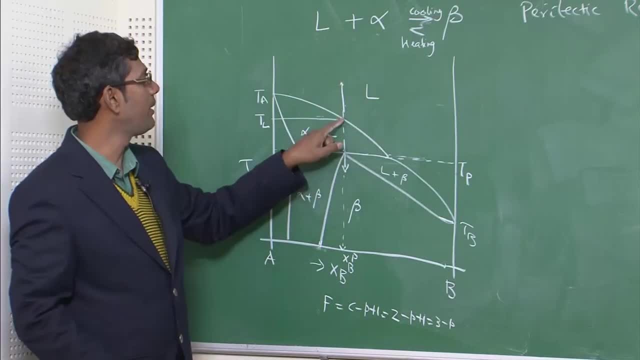 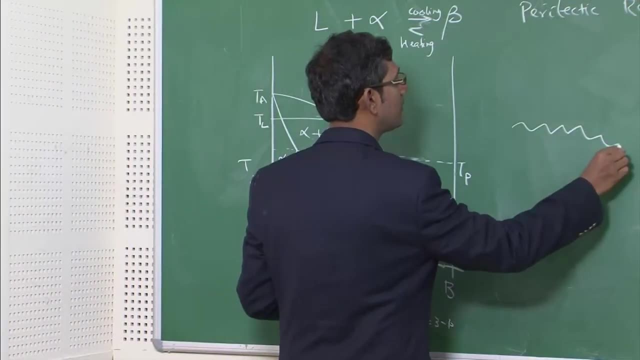 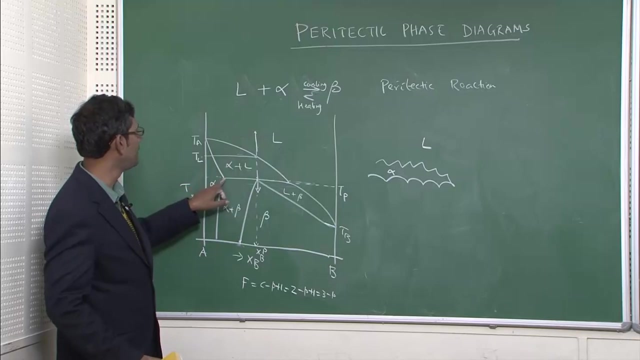 will be liquid. So this is the liquidus. Only below the liquidus, alpha will start forming and alpha will start forming and alpha will grow like a dendrite in the liquid. This is alpha in contact to the liquid. In this temperature between Tl and Tp, alpha will grow in the liquid like a dendrite. okay, 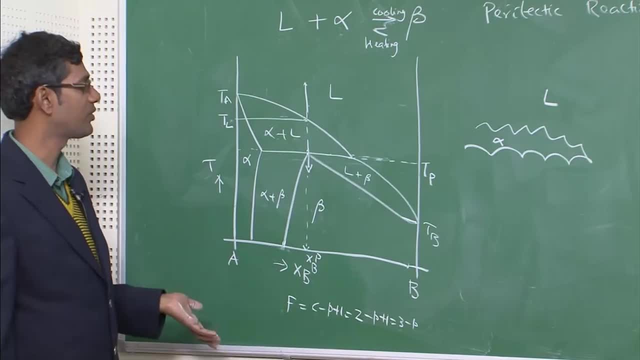 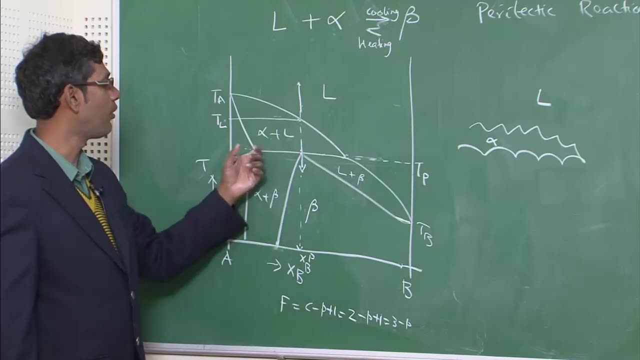 That is because this is the most easily formable shape possible in the liquid state. Now, when alpha, When the temperature of this system is 0,, alpha will start forming and alpha will grow like a dendrite. So the temperature of this system will go down below the Tp, alpha and liquid will react. 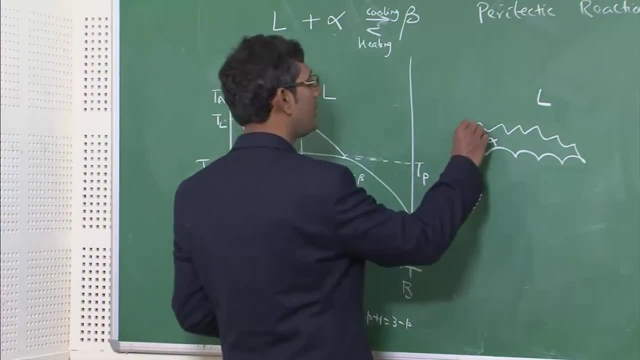 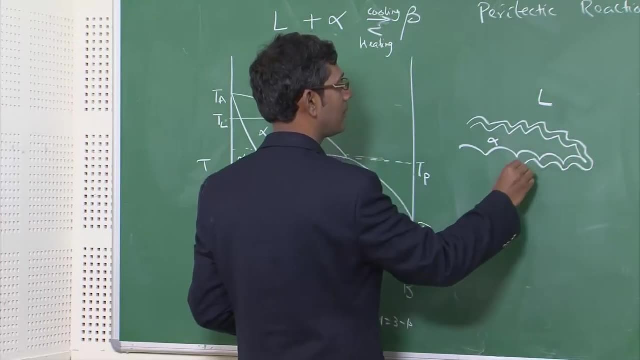 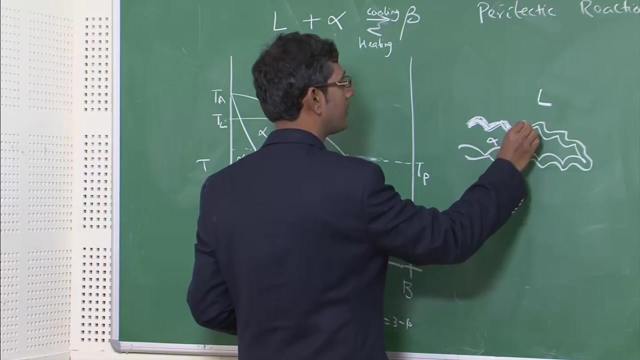 and if they react, they will form beta. How the beta will form: Beta will form on the at the interface between alpha and liquid like a layer. So this is the beta layer which will form in between alpha and liquid. You can clearly see I am marking like a white chalk, using white chalk. 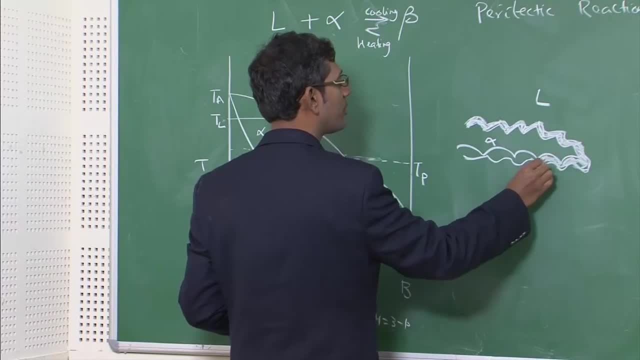 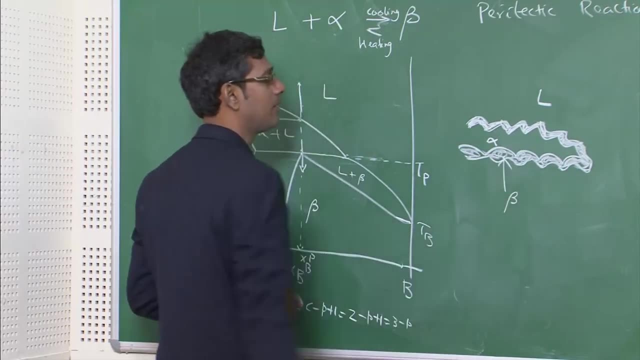 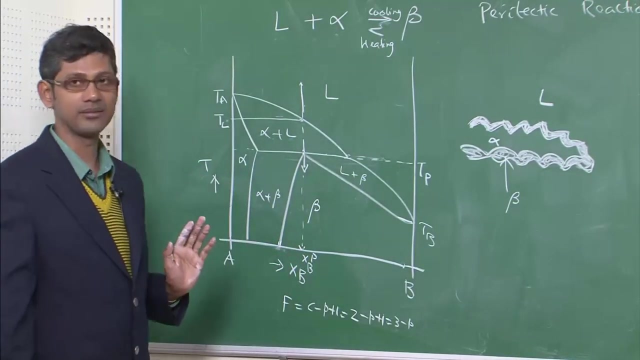 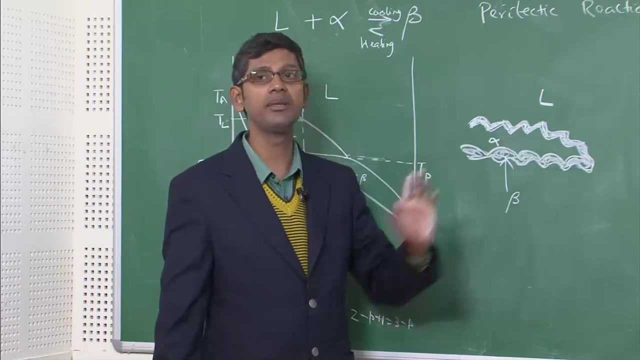 This white chalk has some beautiful layer is beta which has formed because of reaction between alpha and the liquid. so this is beta. So this beta which is formed on the alpha will immediately stop the reaction. why? because as soon as the thin layer of beta forms on the alpha, the contact between alpha and liquid 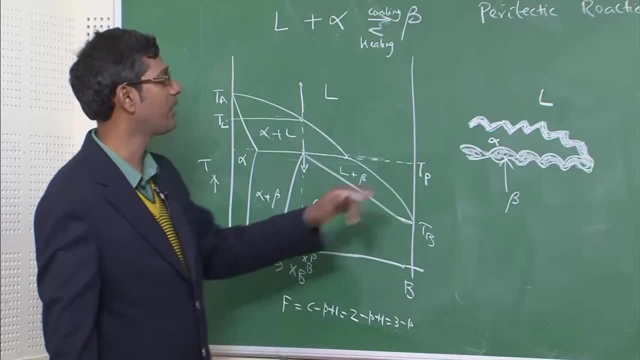 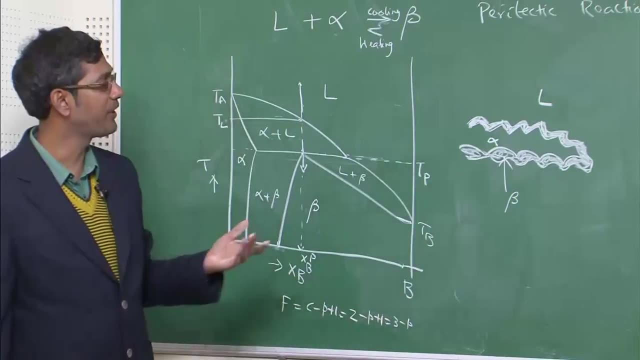 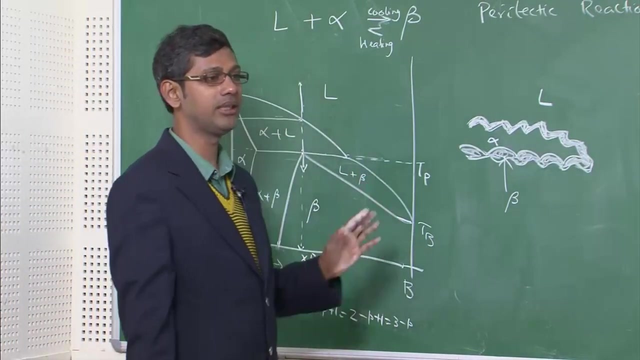 is gone. there is no contact, direct contact, between alpha and liquid. So any further increase of thickness of beta is not because of the p-tree reaction, but by p-tree transformation. What is that? Well, let us little bit dwell on this matter. so, as you see here, SOI form a thin layer on 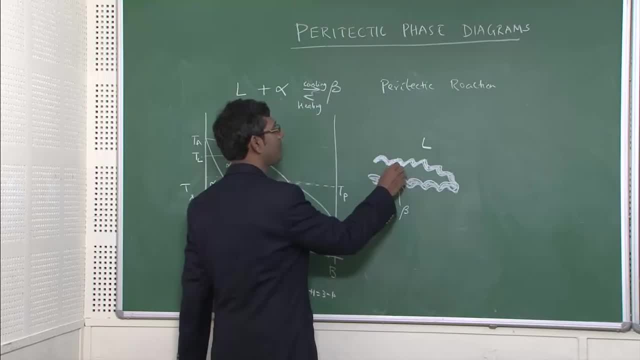 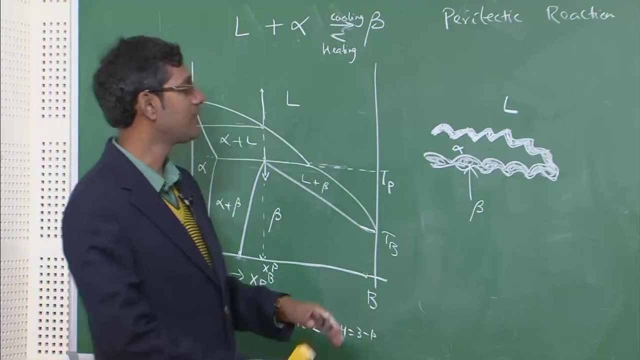 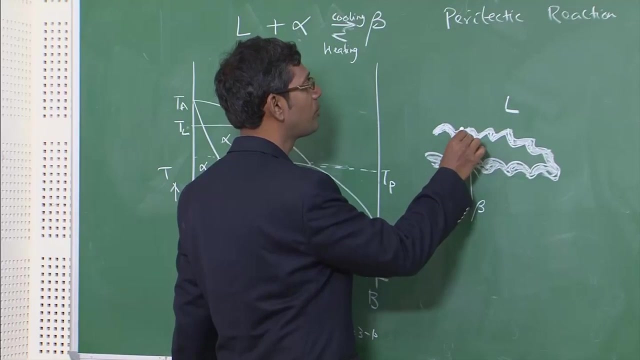 the top of alpha thin layer, so between liquid and alpha. So any kind of contact, Direct contact between alpha and liquid is not there. so the situation for the reaction to proceed or reaction to go further, atoms in the alpha has to diffuse through this layer. 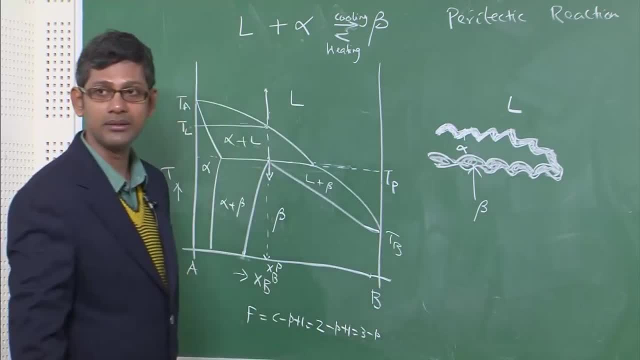 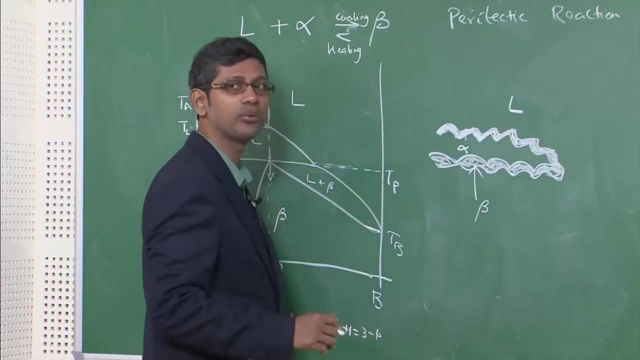 of beta and come in contact with the liquid, because reaction is only possible when there is a contact. otherwise reaction is not possible. and here it is liquid and solid. so therefore direct contact is required. When there is no direct contact, only way it is possible is that atoms in the solid 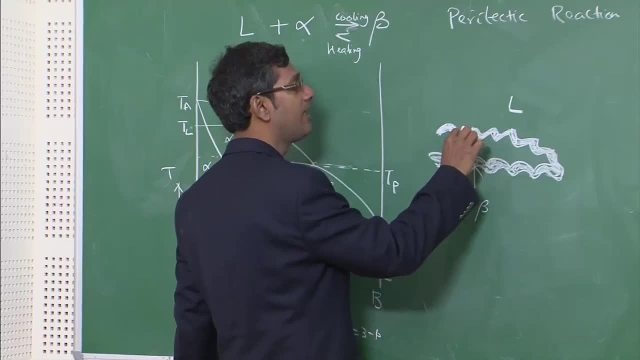 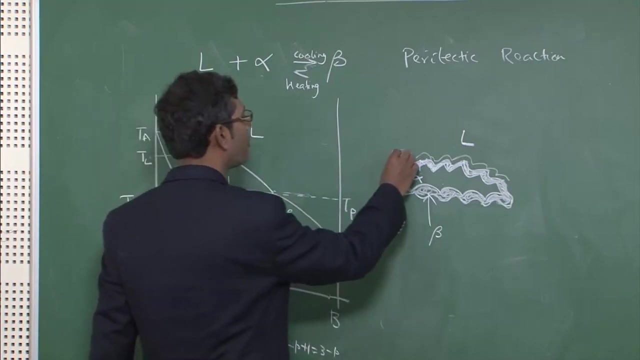 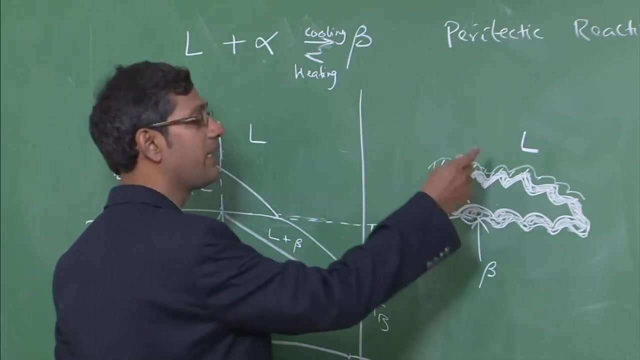 alpha Will diffuse through the layer of beta, come in contact with the liquid, and when it comes in contact with the liquid it forms another layer of beta. okay, Suppose this is the layer layer of beta forms. So as it forms another layer of beta, the thickness of the beta will increase. so for 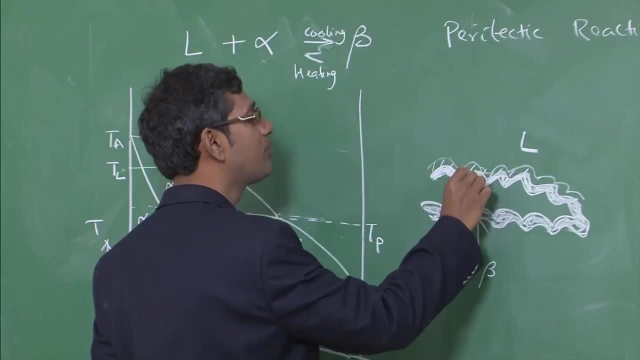 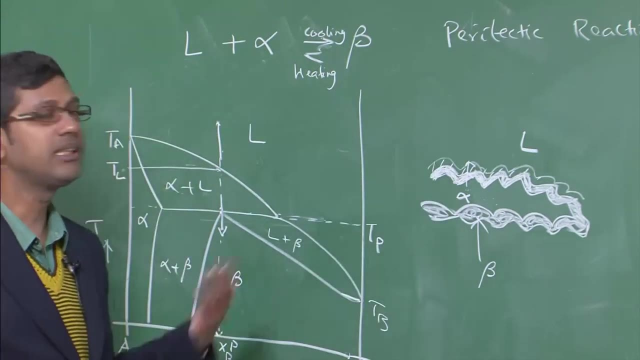 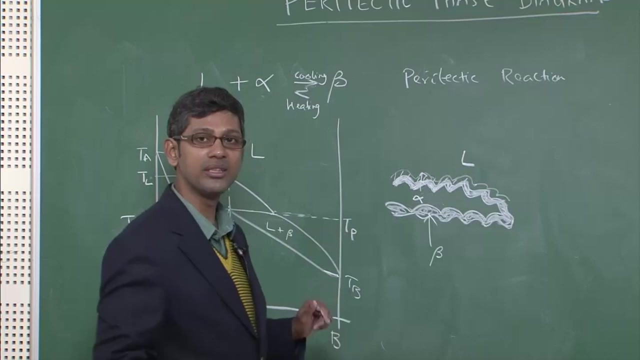 any further reactions. atoms in the alpha again has to diffuse through this whole layer, come in contact with liquid And the diffusion distance each time is increasing. Why? because thickness of the beta layer is increasing. As the diffusion distance increases, the time required is also increased. because I know 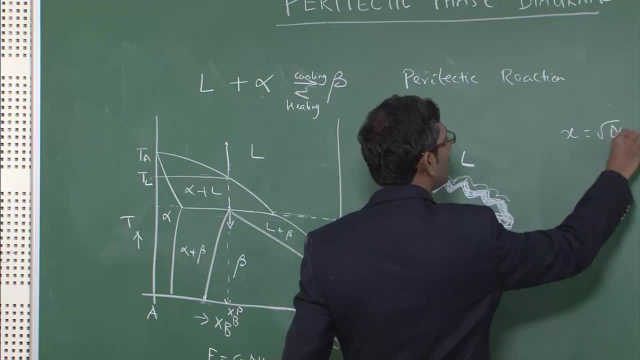 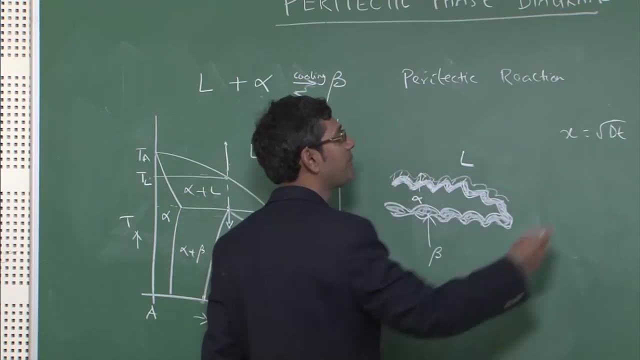 that distance is equal to do DT, where X is the distance, that is, the time, and D is a diffusivity. So as we increase X, D is remaining constant. same time T increases. so therefore, as the time increases, Time T increases. Time D times, Dt, time t increases. so therefore, as the time increases, you need a dough. you get a whole protocol of map and you draw some fifth formula, Duhb, you actually write down this one- yeah, I was talking about it earlier in the class- and then also, this is the principle of V. I am 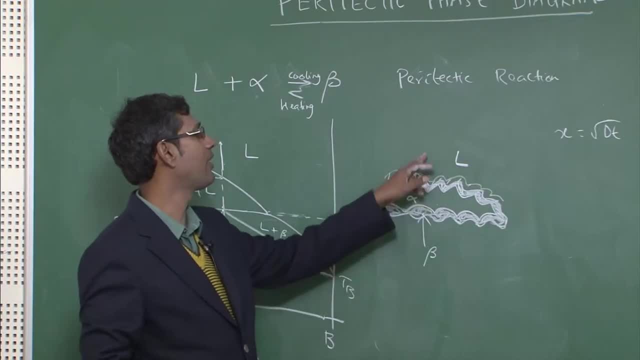 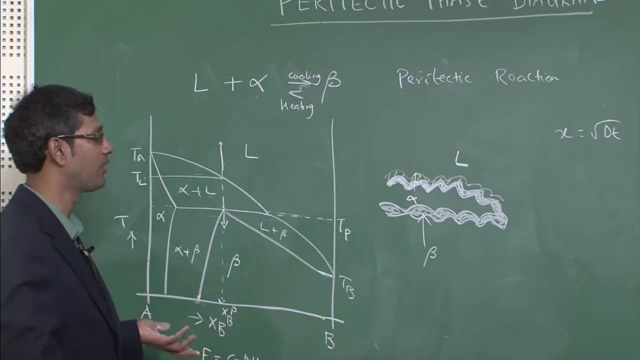 gonna go in further class. more time for the atoms to diffuse, from alpha to come in contact liquid, and after some time this time will be very large. so therefore no further diffusion is possible and under such a situations you will always have some left over alpha in the microstructure, which 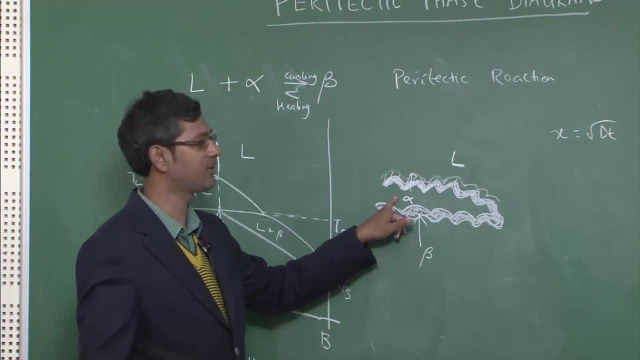 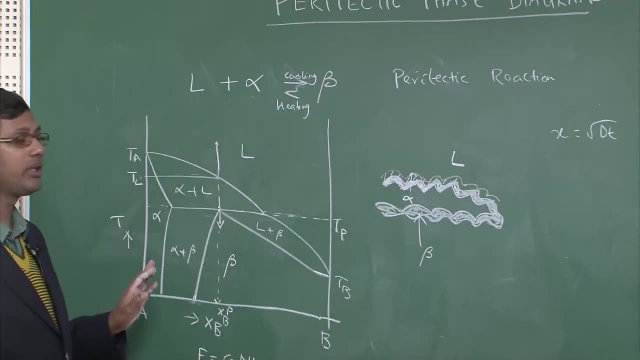 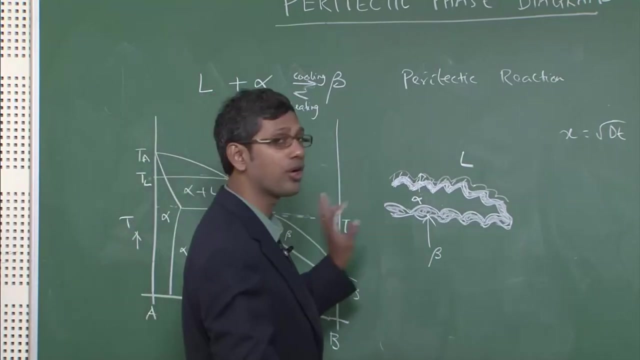 you cannot help. There will always some left over alpha present in the microstructure because incomplete reaction- this is the problem with all pated reaction. pated reaction under normal cooling conditions will never get completed and that creates lot of problem in the industry. okay, which? 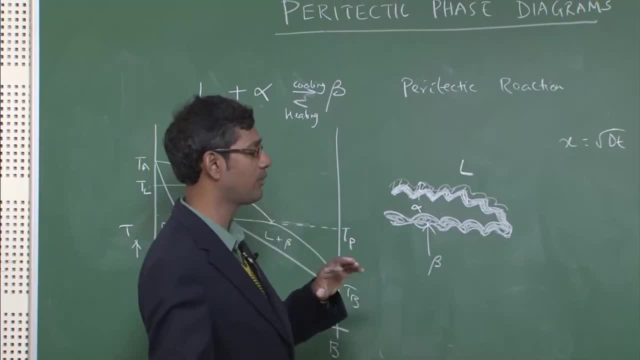 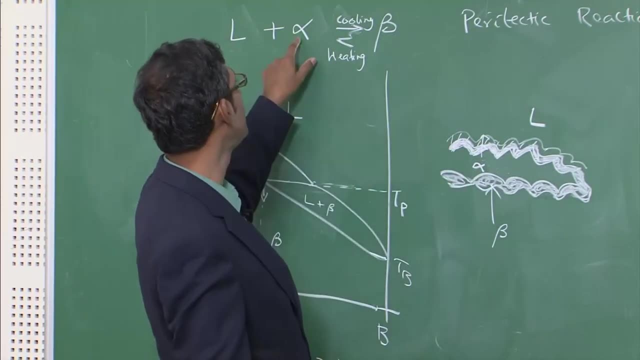 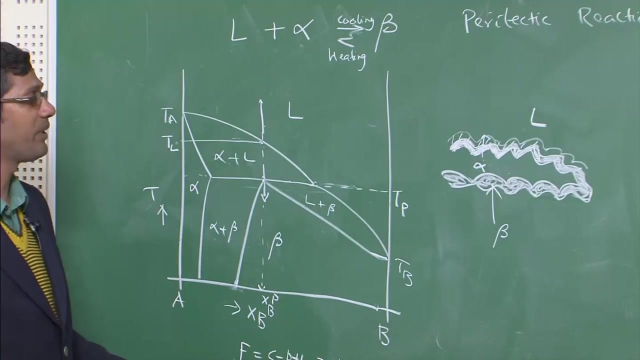 will discuss one or two case studies, will discuss in the whole class, in one of the classes where I will show you that retaining this phase alpha, which is known as, which is this phase- at a temperature lower than the previous temperature can create lot of problems in the properties of the material. 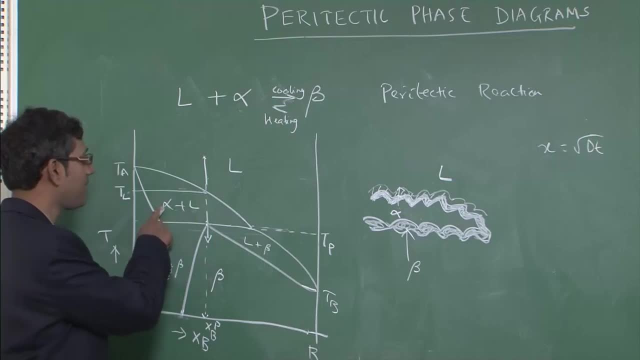 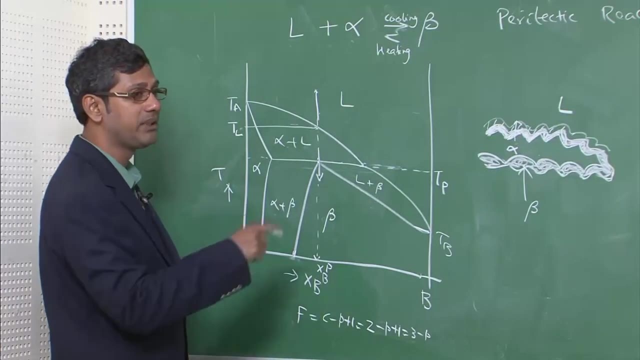 So, as you see here, alpha is known as pro eutectic, Pro eutectic phase, just like eutectic. I have discussed pro pated eutectic phase because it forms before the pated reaction and beta is known as the pated eutectic phase and because 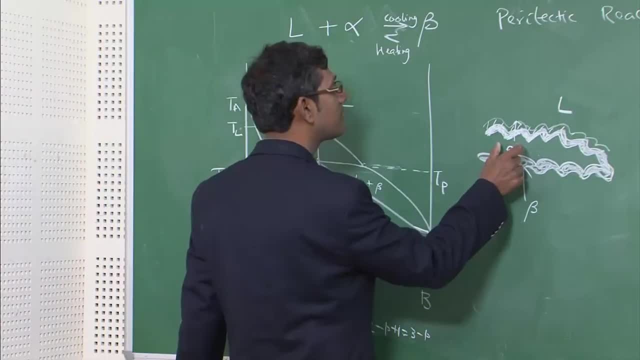 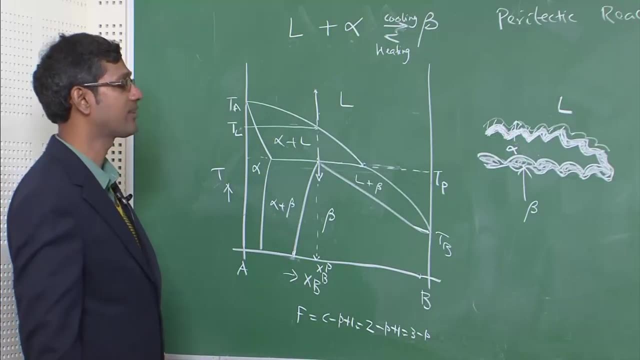 it forms after the pated reaction. So you will have always pro pated eutectic phase alpha retained in the microstructure because of incomplete reactions, of pated eutectic reactions of this kind. So because of this it can create all kinds of problem, as I told you. 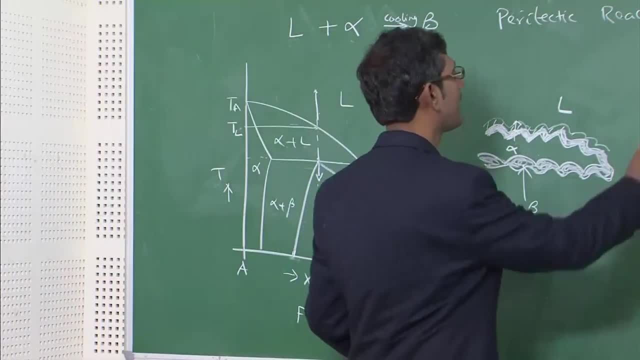 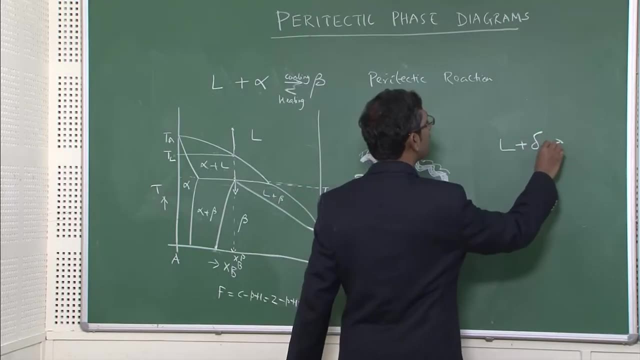 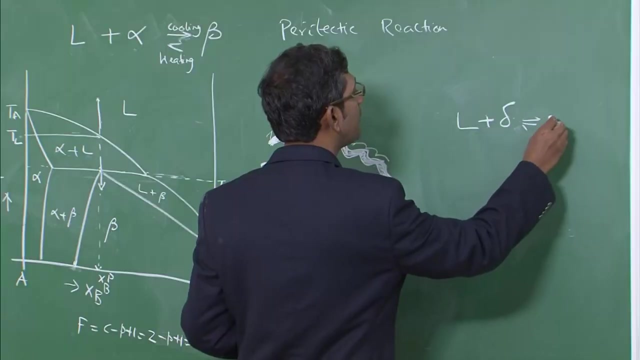 Suppose. let me just explain to you the pated reaction which is present in the iron carbon phase diagram. Pated reaction present in the iron carbon phase diagram can be written like this: liquid reacting with delta, iron or delta, rather okay- reacting with liquid and produce gamma. 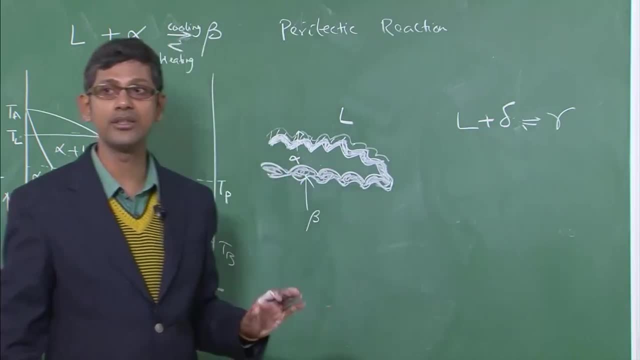 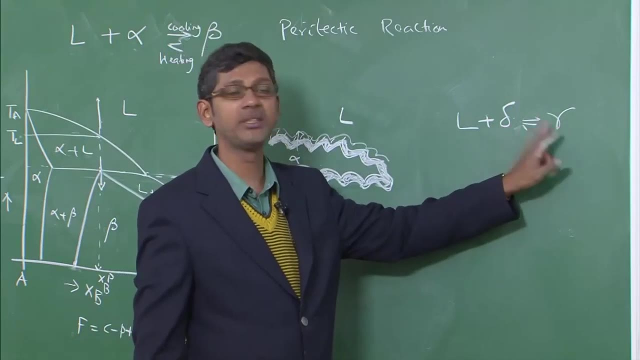 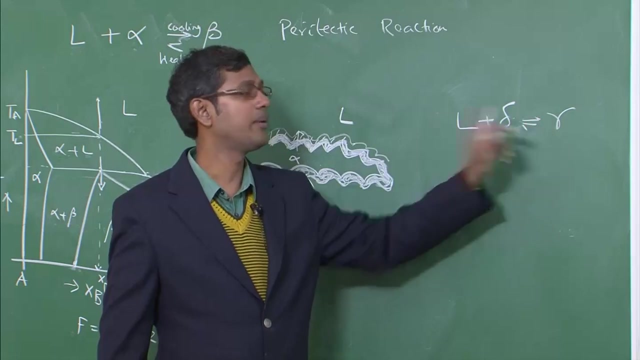 As you know, that iron has 3 phases: alpha, beta and delta in the normal pressure, and delta is a BCC phase, BCC iron and gamma is a BCC phase. Okay, Okay, So alpha is also BCC phase. So now, in this reaction, liquid plus delta going to gamma, same thing will happen and 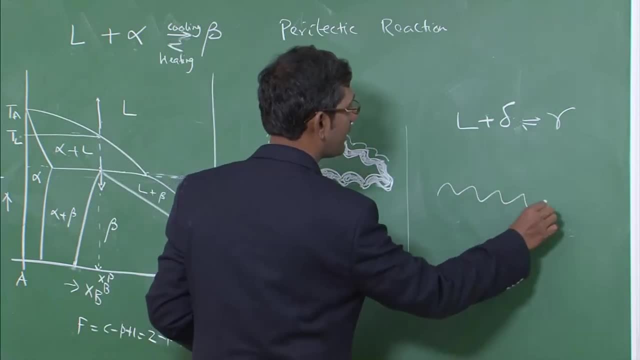 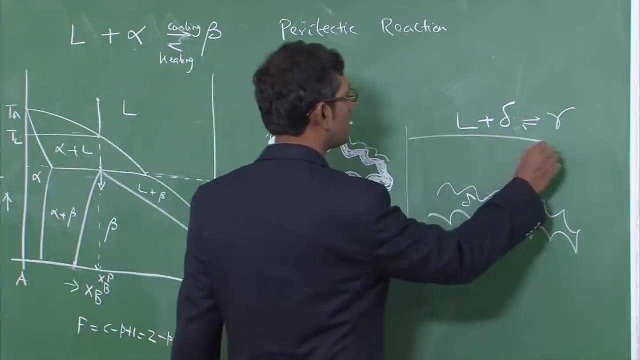 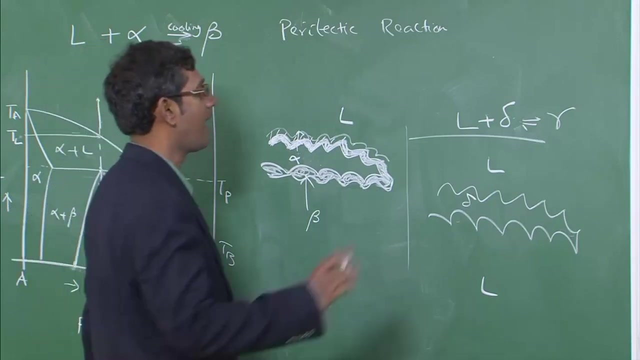 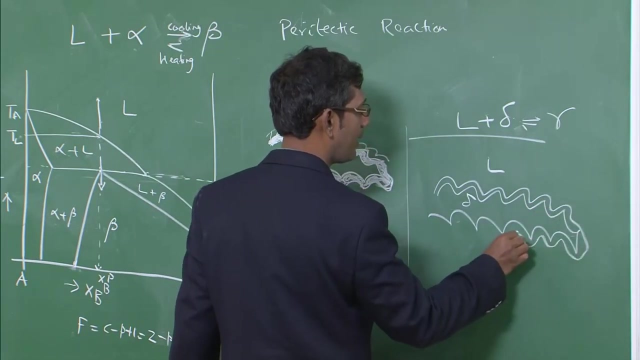 I will draw it again here. So I have a delta dendrite coming in the contact to the liquid and as the reaction happens. this reaction happens at 1394 degree Celsius temperature. As the reaction happens, You can see here that gamma will form like a layer, like a layer around delta. 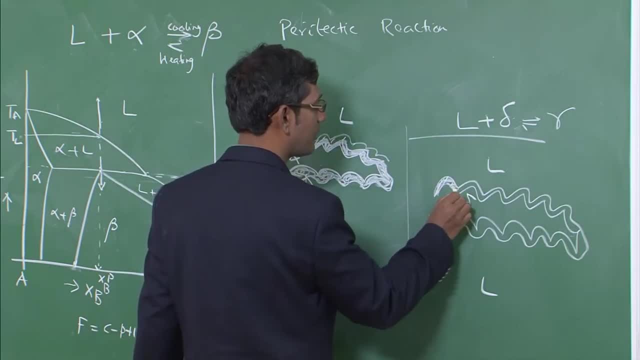 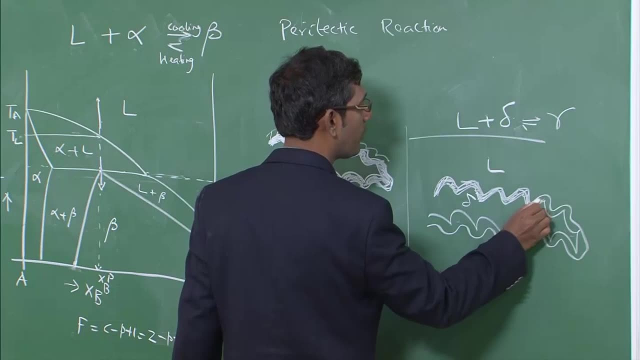 This is gamma. It is better to mark by a chalk gamma. and as time goes, gamma layer will increase one by one, but it cannot be consumed. the full delta, it cannot consume the full delta. delta will retain, Delta will remain, rather, in the microstructure. 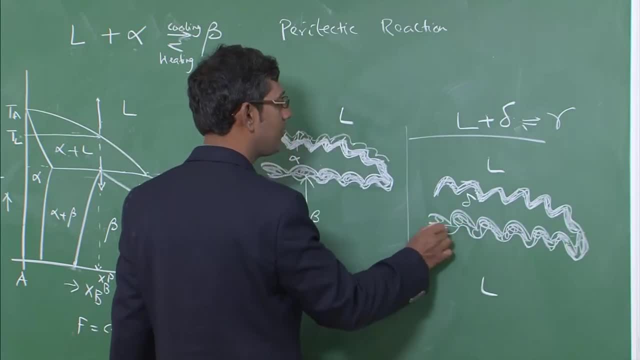 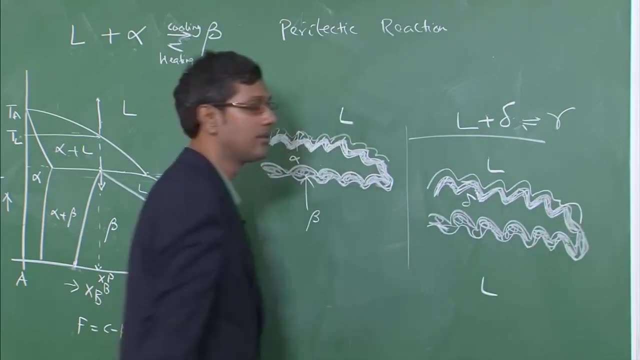 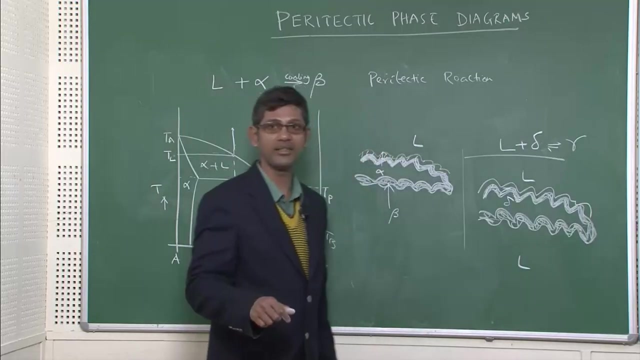 Okay, So another, as you give more time, another layer of gamma will form, but you know, delta will retain because of the nature of the reaction. Now suppose this whole microstructure is solidified and you are retaining it at your at room temperature. At room temperature delta is not stable, but gamma is stable. gamma will retain, they remain. 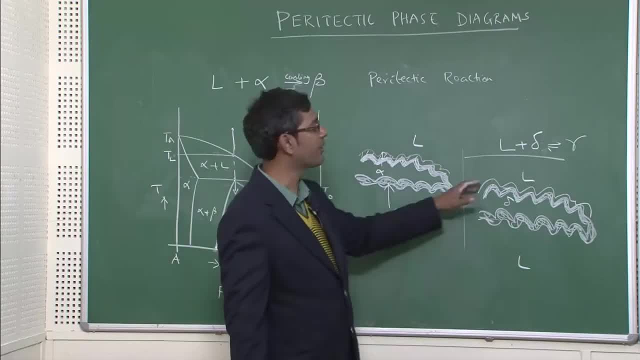 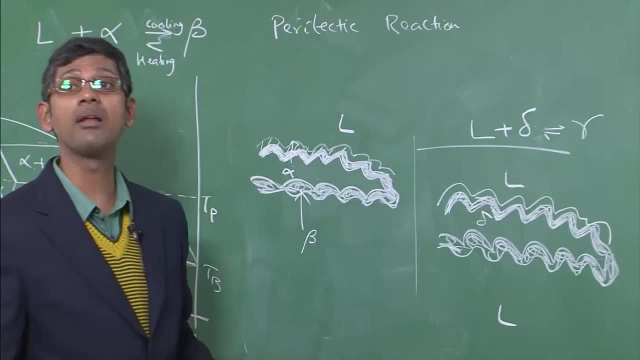 there. Delta or gamma is also not stable in here. But gamma will undergo The other reaction to form pearlite in here, but delta is not stable at room temperature. Delta will form alpha iron at room temperature or it may not form because of pressure effect. 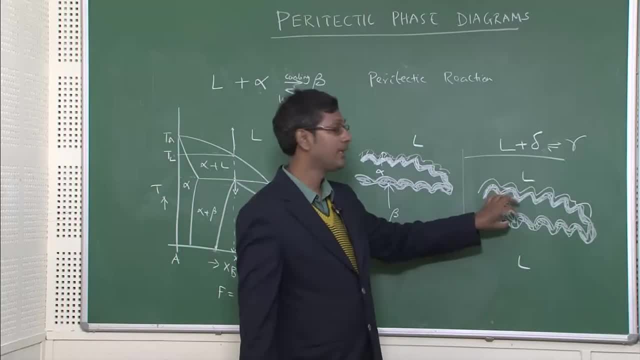 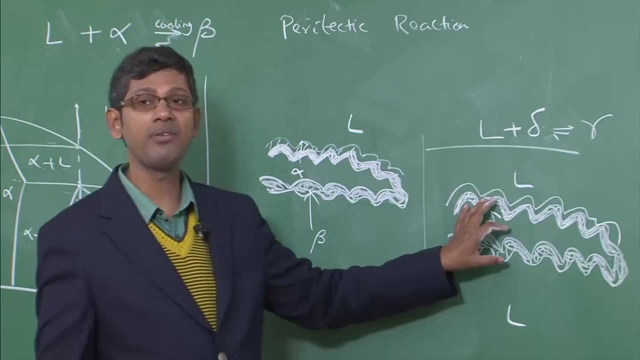 Whatever it is this has, this will create lot of problem in the, in the, in the final properties of the material, because you ultimately finally in a steel. you what you want is alpha as a primary phase and pearlite. You do not want anything else. Okay, 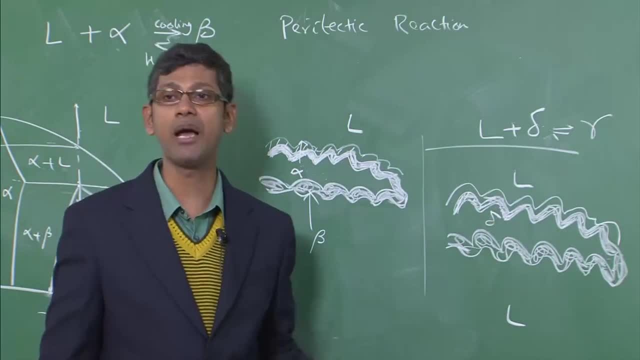 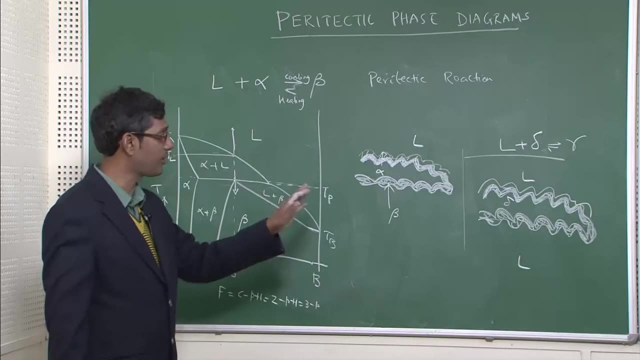 For the normal steels. So you can see here this: this: this happens only with very low carbon concentration in the steel and because of very low carbon concentration steel, these categories of steels are basically stainless steel and therefore this is a very critical problem in the stainless steel. 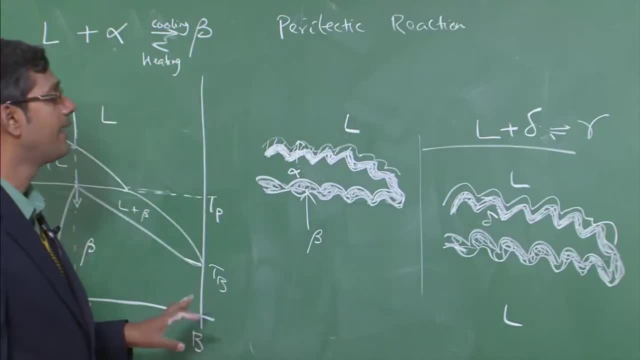 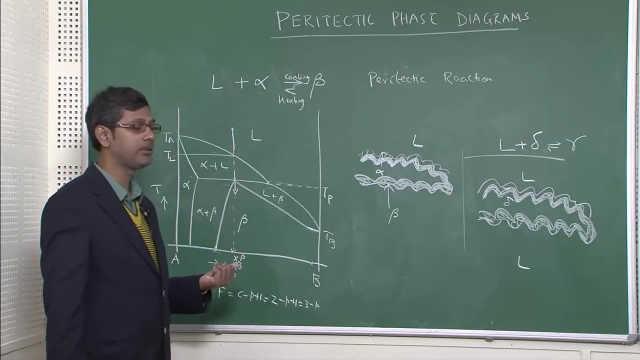 In all stainless steel you can have this, this problem, and in fact there are other stainless steel contain iron, chromium and nickel than carbon, So therefore they are actually chromium, can segregate Okay And reacts with carbides and form chromium carbides. there are additional problem, which 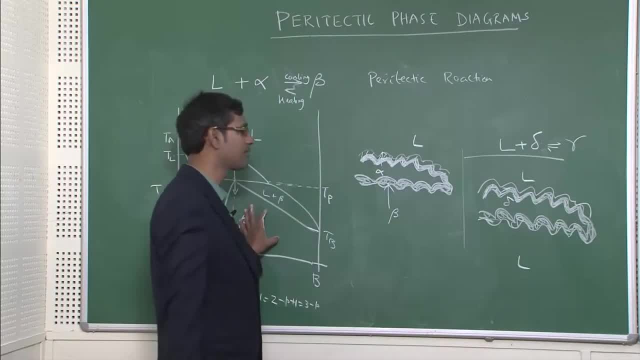 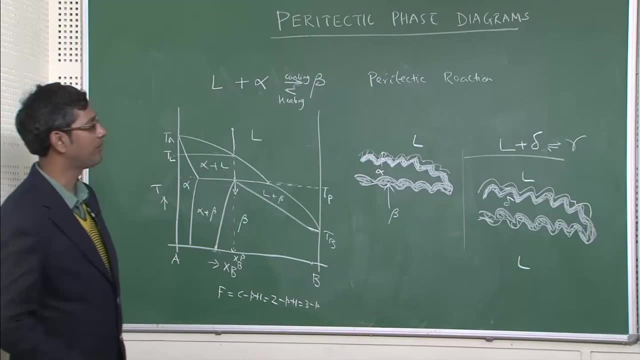 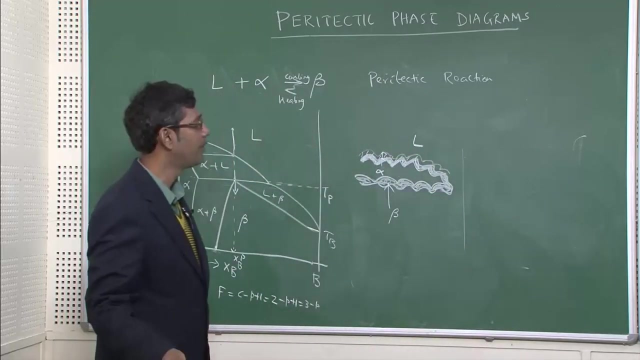 you will discuss later. but from the perspective of the pay to reaction, you understand that this is can go, can create problem. another example, I will give it to you, which is very interesting: all the headphones nowadays used for iPod, iPad or mobile phones has a very small magnet into the, into the headphone, and these magnets actually very strong and most 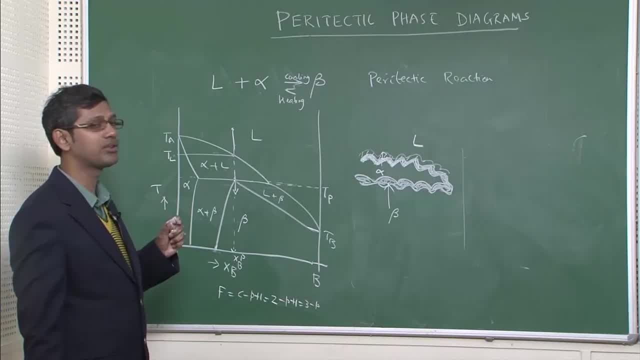 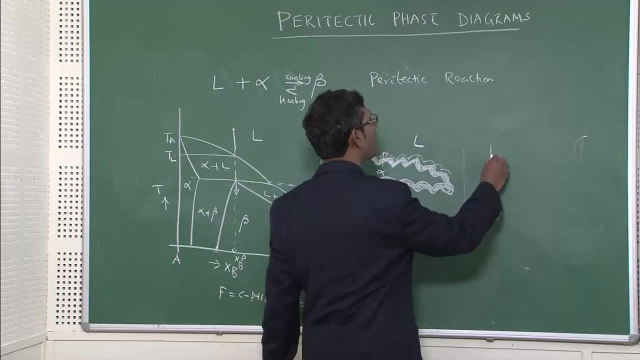 of these magnets come from China, and China has the largest source of this material. that is why they have the monopoly: almost 96% market share is by China. This magnets actually are this type. it contains titanium, neodymium, iron and boron. 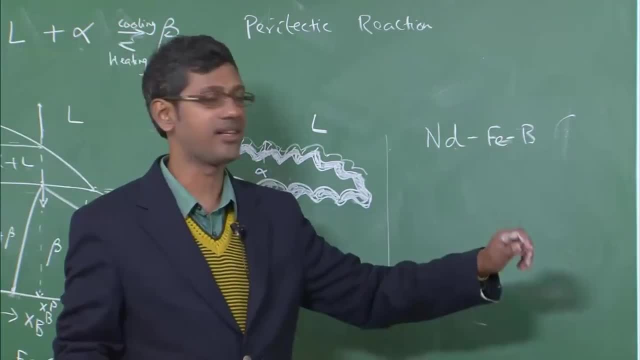 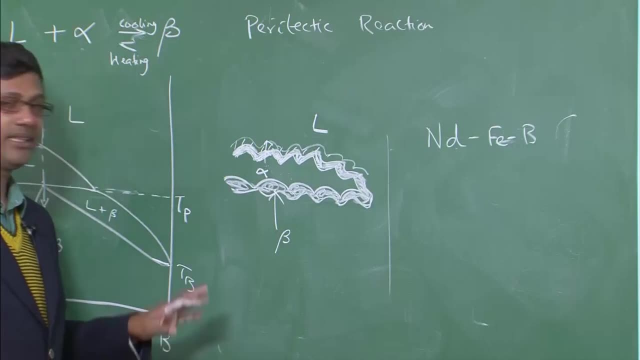 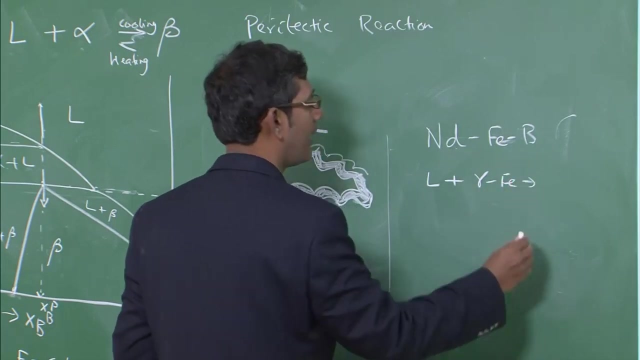 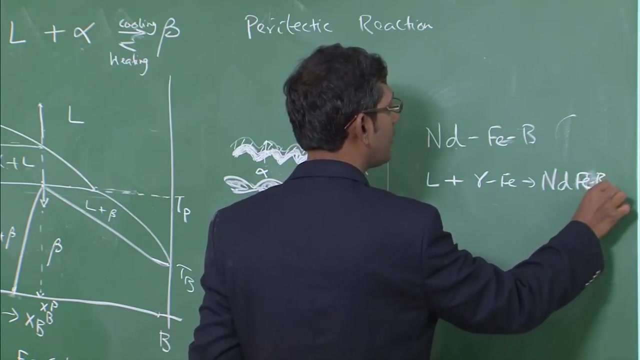 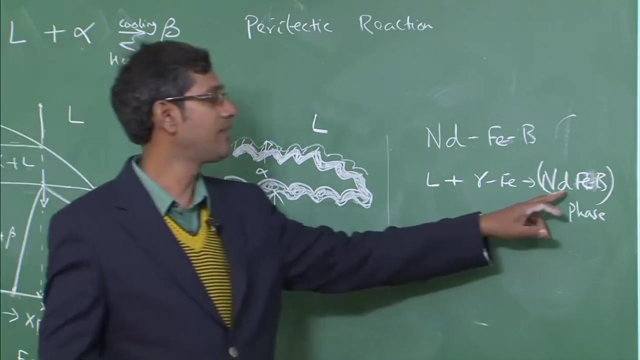 Okay, and iron boron most of the countries has. what you do not have is the neodymium. Neodymium is a rare earth metal. so these alloys, actually these alloys actually undergo a pay to reaction Liquid with gamma iron reacts and form a NDFEB, NDFEB phase. these alloy forms, remember this- 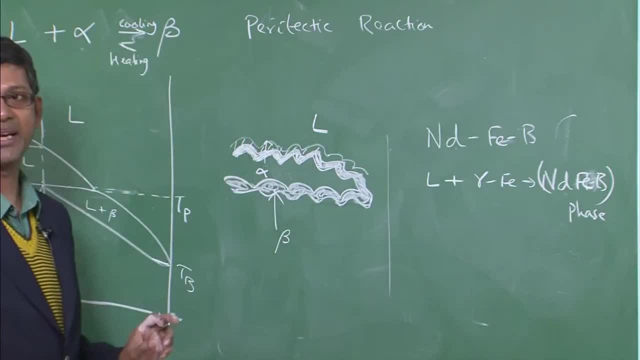 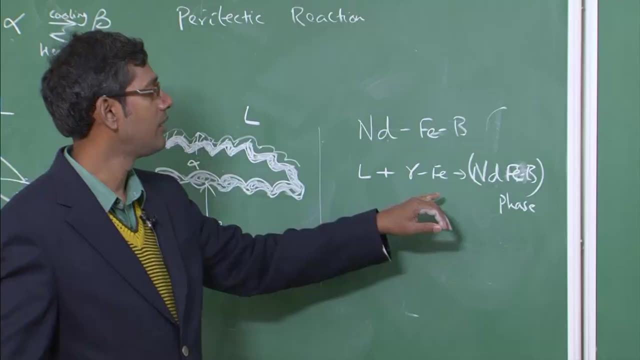 is the magnetic phase. all the speakers actually hard magnets which we use to listen music or listen, you know, all kinds of other things. So like we can use for other problems, Okay, For other purpose also. they- this is the magnetic phase. this is a hard magnetic phase. 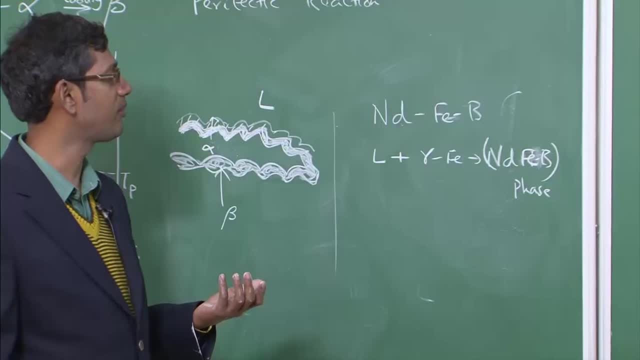 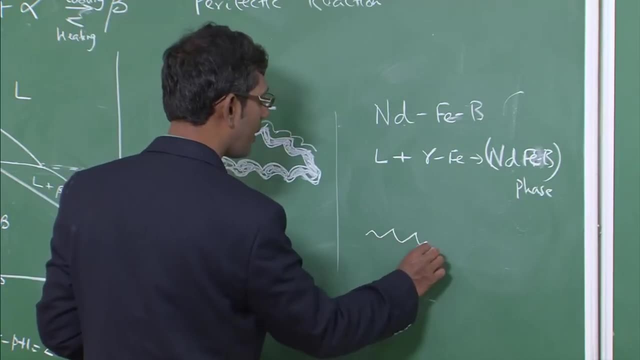 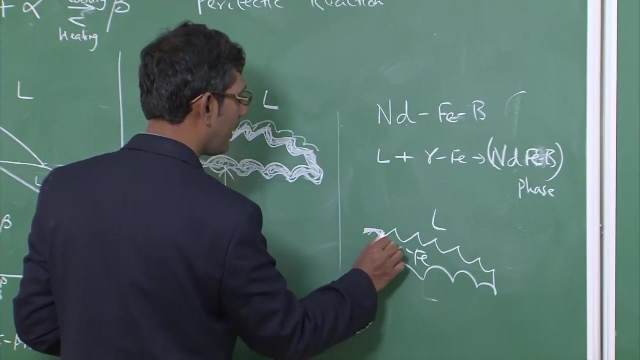 So if you want to use, increase this strength of that, you want to have more of this phase. but as you see here, because of this pay to reaction, you will have from gamma phase present gamma iron liquid and then this phase will form on the layer between gamma and liquid. 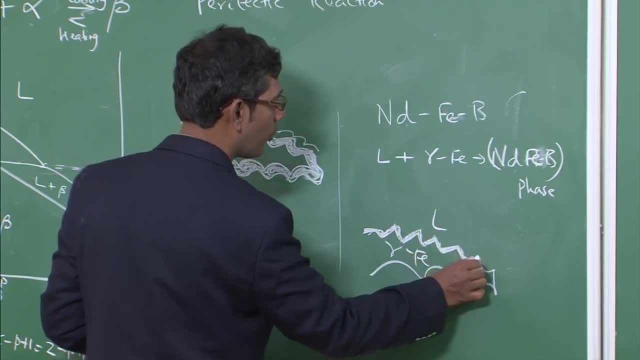 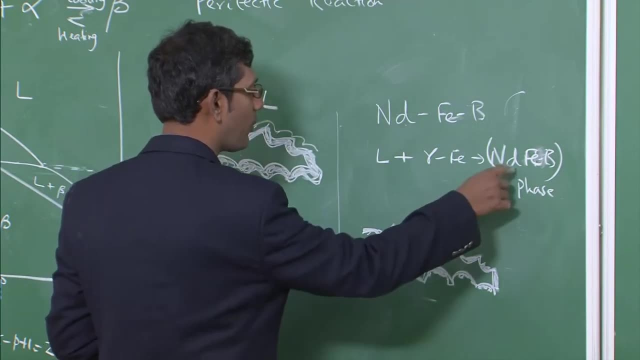 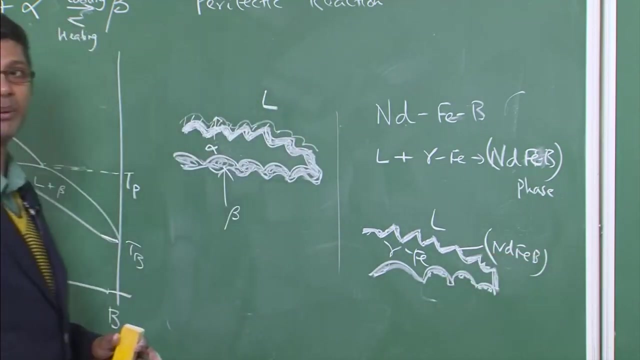 like this, but, as an engineer, what you want? You want this. This is because the hard property, hard magnetic property, is provided by this. this is what is this? NDFEB phase? okay, ND12FEB actually. so, because of that, you want to have maximization. 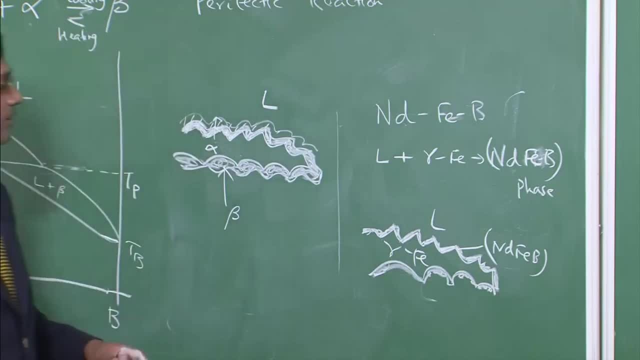 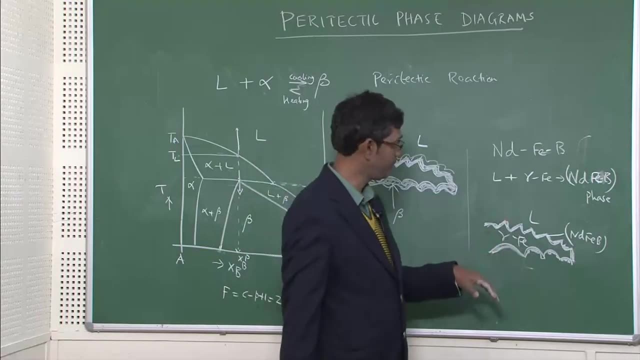 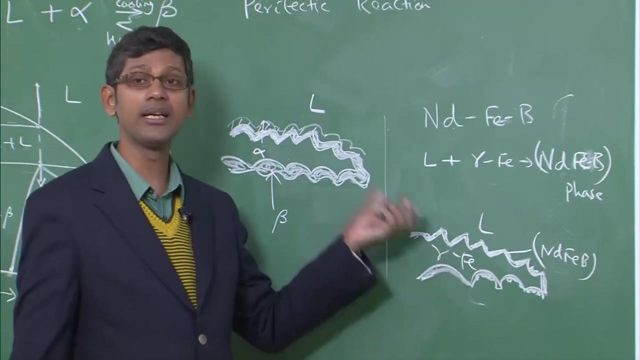 of these particular phase in the microstructure, because this will give you more energy product or more stronger magnets, hard magnets. but it will never happen because by pay to reaction there will be some gamma left over. Okay, So this gamma will create problem, because if this gamma actually later on room temperature, 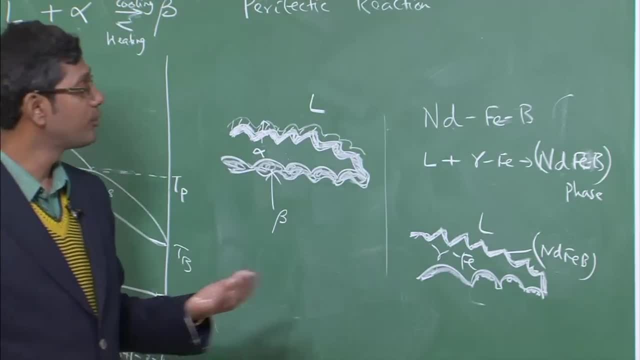 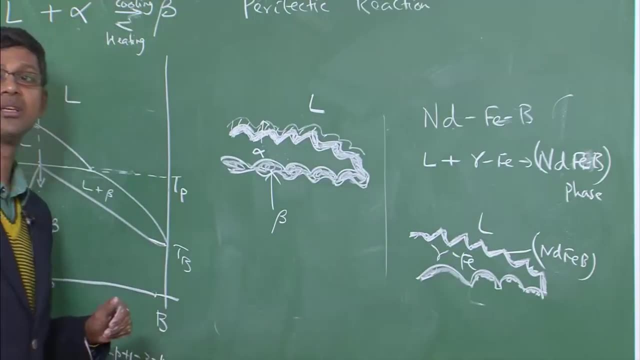 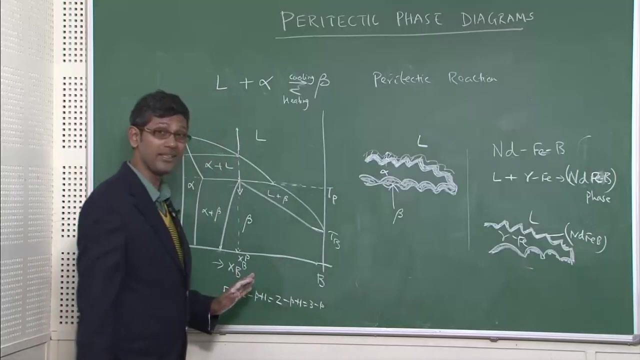 will transform to alpha iron, and alpha iron is a soft magnet. So if you have a- you know- soft magnet inside this, at center of the hard magnet, this will reduce the strength of the hard magnet. So therefore there must be some solution to that. So what I am telling you is that pay to reaction creates problem in the, in the, in the industry. 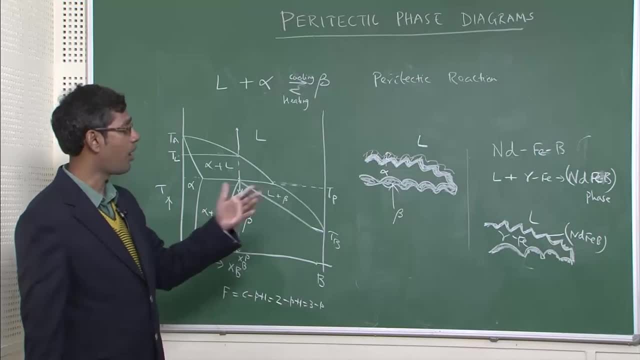 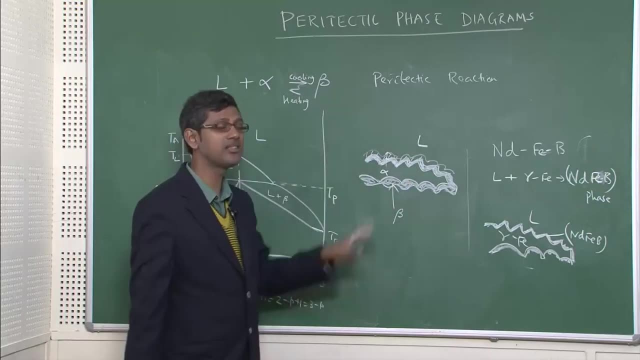 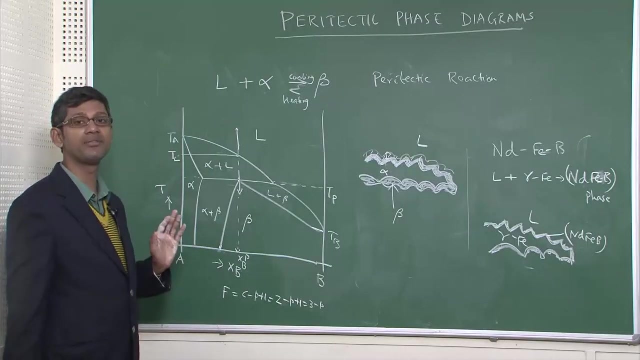 actually all this pay to reaction like a stainless steel, I told you all, in in the magnets it creates problem and the main problem- arginine form- is nature of the reaction. the reaction is such that it can creates problem which we have to deal with it, and that is why it is important to understand the patectic phase. 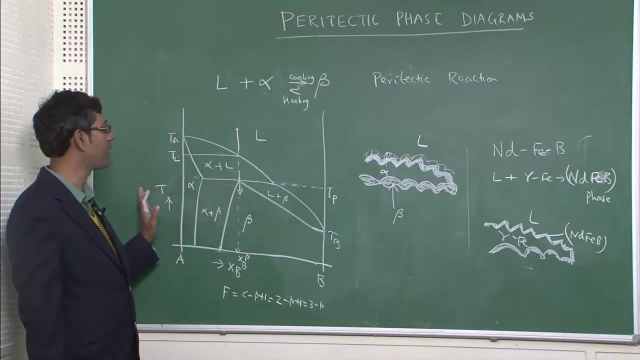 diagrams very nicely. if you do not know the patectic phase diagram very nicely, you cannot control. to give you a hint, because those of you who are intelligent enough or able to understand my lectures nicely, you can actually bypass this patectic reaction. What is the meaning of bypassing? 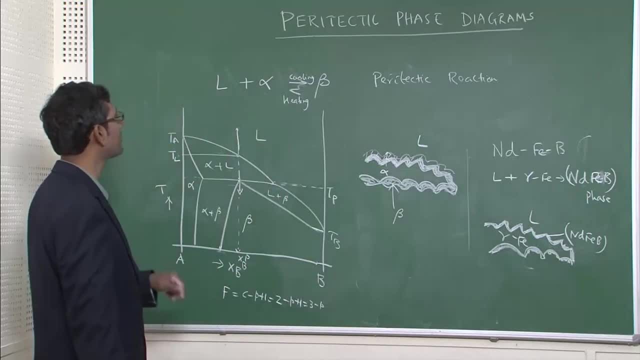 What is the meaning of bypassing? What is the meaning of bypass, which I will discuss detail matter next class. but I am just giving you a hint. you can actually directly form beta, form liquid instead of alpha. that means you can actually, you do not need alpha to form beta. normal classical pateotic reactions. 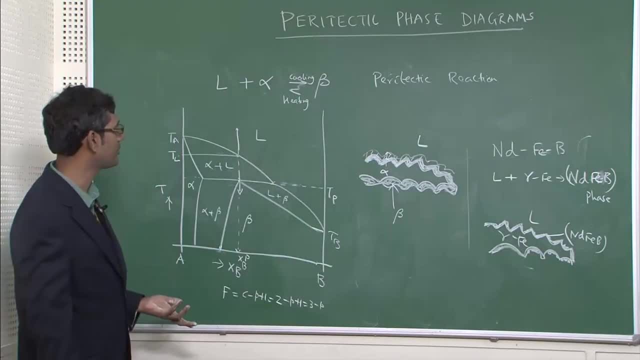 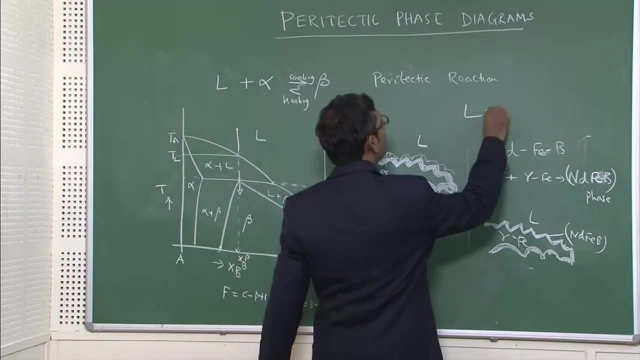 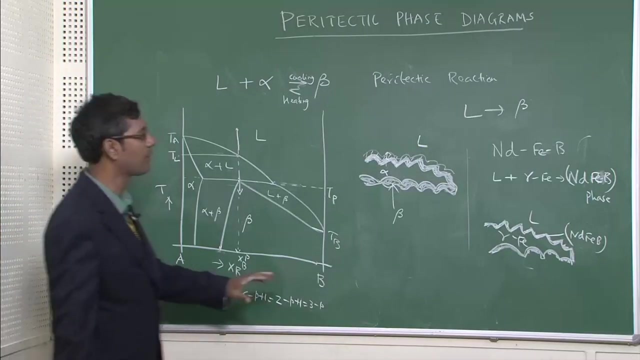 you need alpha to form beta. liquid is anywhere present in the microstructure, in the, in the alloys, So you do not need alpha to form beta. so you can actually directly go from liquid to beta, If this is possible. if this, I can do it by under cooling the alloy. what will happen? because 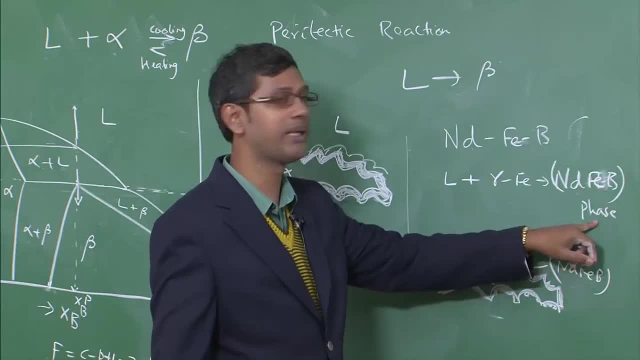 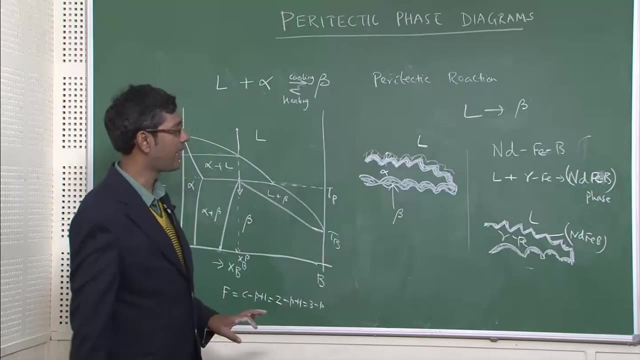 there is no gamma iron present, liquid directly NDBFE B phase will form on the liquid. there is no soft phase at the center of the of this magnet, of the hard magnet, and we can produce harder magnet. this is a technology which has been mastered, which has been rather developed. 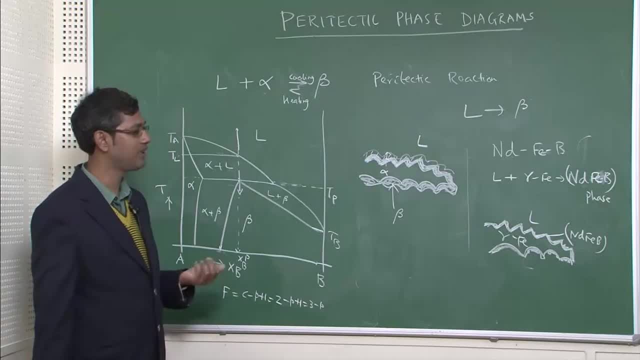 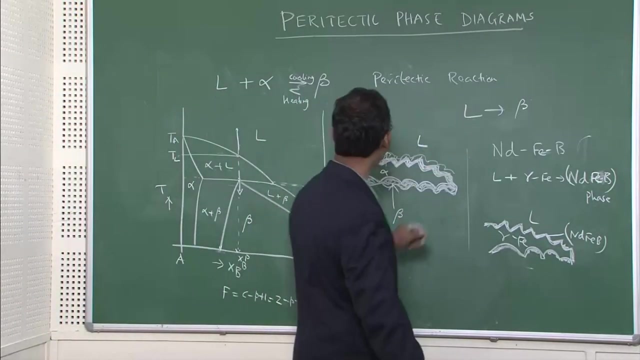 and mastered by the, by the people in the world, Especially the China, in China, and that is why they could make very strong magnets. and those magnets actually are very, very useful and can be utilized for many applications. that is what is done normally in all the things. if you under cool the liquid strongly, you